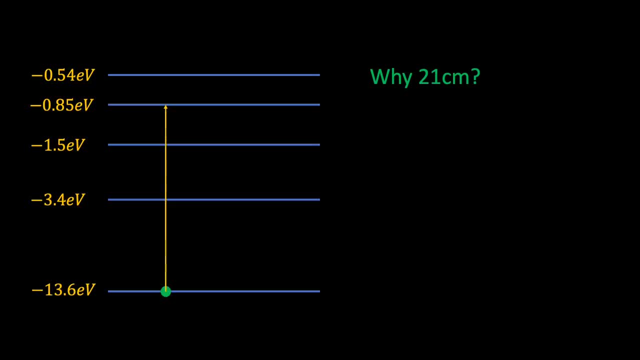 energy level. The electron is able to return to the ground state by jumping from a higher to lower energy level by releasing a photon of energy. The energy of the photon determines the wavelength of the light emitted. In the case of hydrogen atom, the transition that causes the 21 centimeter microwave radiation is: 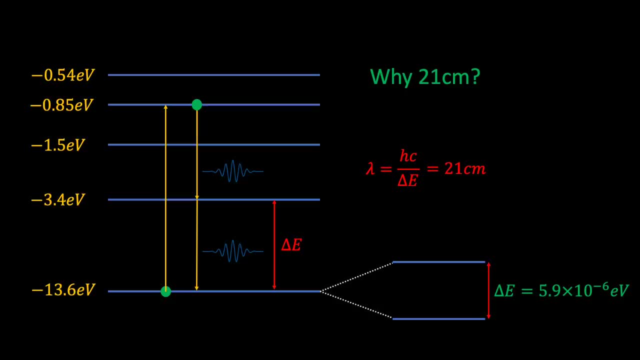 between the two levels of the hydrogen ground state, which is slightly split by the interaction between electron and nuclear spin. The splitting is known as hyperfine structure, and the tiny difference in energy between the two split levels is what causes the emission of the 21 centimeter microwave. 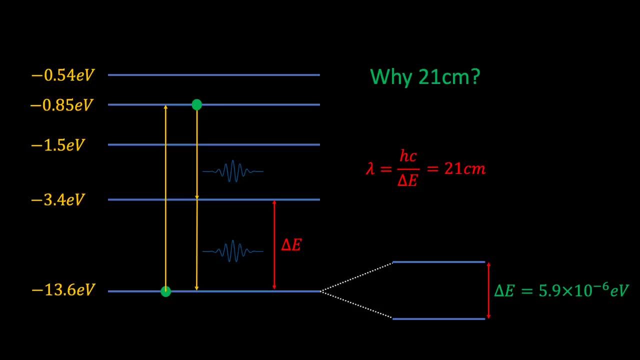 radiation, And it was because of the relative energy of the hydrogen atom that the energy of the hydrogen atom is generated. It is the relative abundance of hydrogen in our own galaxy that Penzias and Wilson expected the dominant wavelength of microwave radiation to be 21 centimeters. Now it turns out that this kind of measurement is very 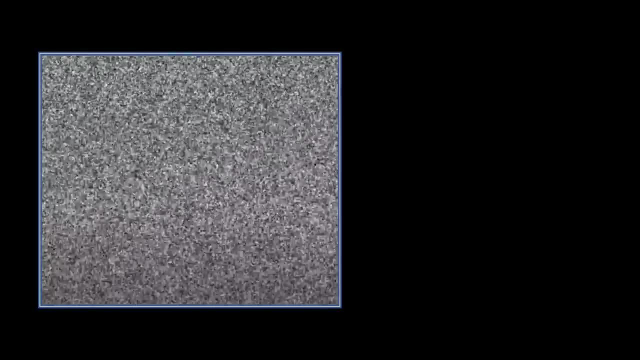 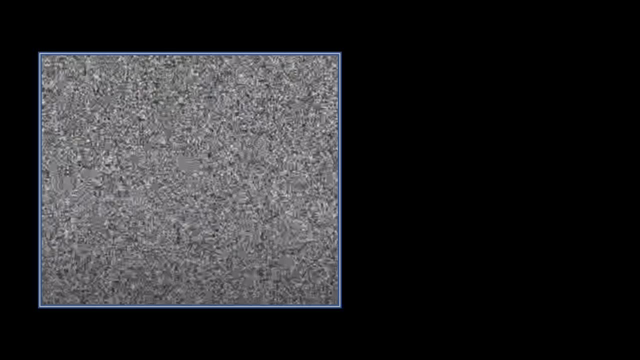 challenging. The microwaves for our own galaxy form a kind of static, much like the static you see when tuning an old analog television or radio. Unfortunately, this static noise is not easily distinguished from the inevitable electrical noise that's caused by the random motion of electrons within the 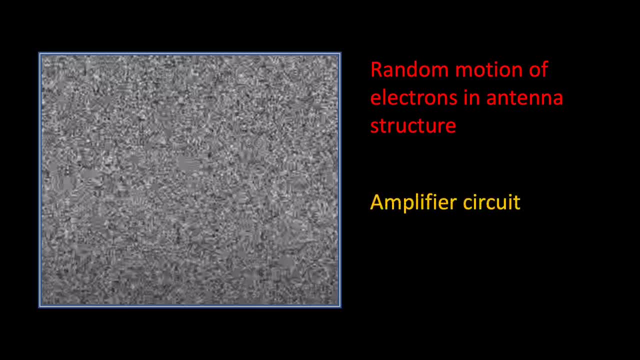 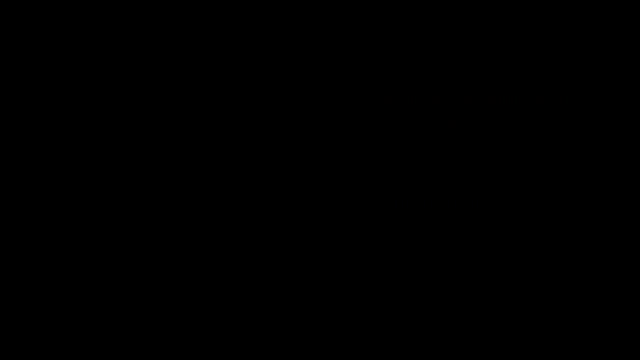 structure of the antenna or the circuits within the amplifier of the detector. Furthermore, there will also be a small amount of static noise picked up by the antenna from the Earth's atmosphere, and all of these need to be accounted for when making a measurement. Now, if you're using the telescope to 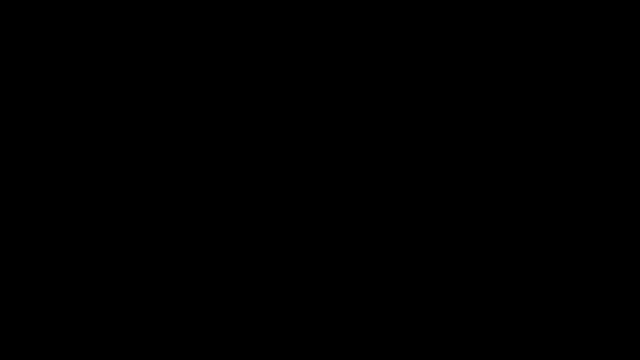 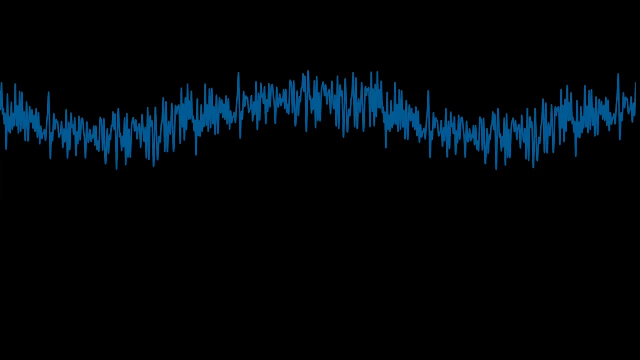 study a small localized source of radiation such as a star, then you can point the antenna at the star, collect the signal, then point the antenna away from the star at an empty region of space and collect the background noise signal. If you then compare the two signals and look at the difference between the two, 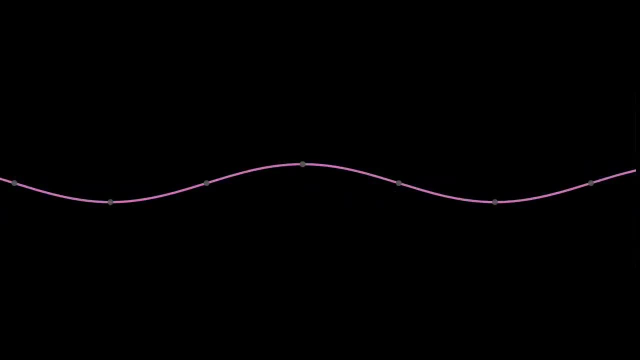 measurements, you can cancel off the noise and recover the pure signal from the source. The reason this works is because any noise originating from the antenna structure, amplifier circuits or from the Earth's atmosphere will be the same, whether the antenna is pointed at the source or an empty patch of sky and 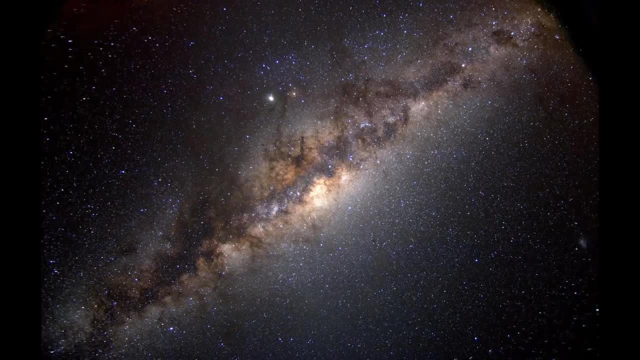 so you can cancel it when the two signals are compared. However, the difficulty for Penzias and Wilson was the fact that they were trying to measure the signal coming from our own galaxy, which we are inside, and so, in effect, they were measuring the signal from the sky itself, making it very difficult to 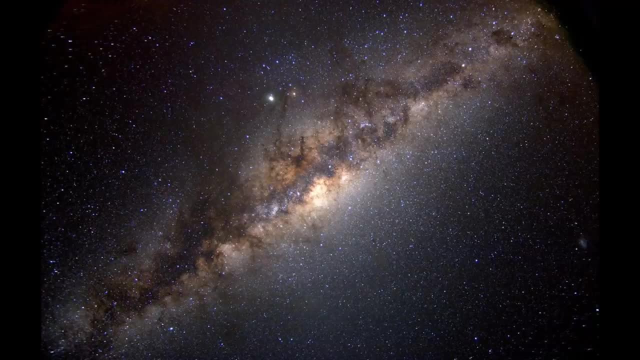 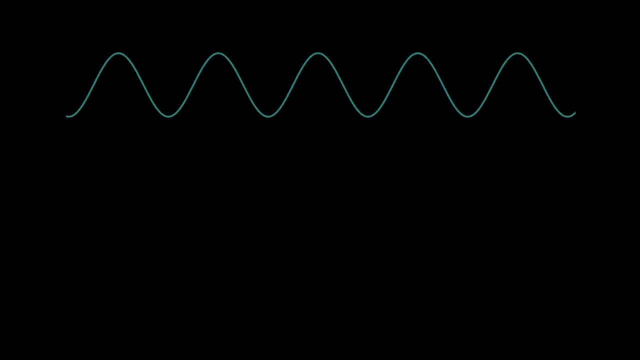 subtract off the noise, because it's difficult to know what is and isn't noise. It was therefore vitally important for Penzias and Wilson to carefully calibrate their telescope and identify and minimize all electrical noise produced in the antenna receiving system, In order to study the noise produced by. 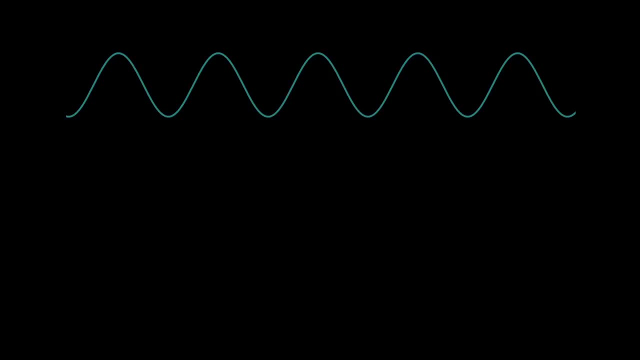 the antenna structure. they ran a series of observations at a relative short wavelength of 7.35 centimeters, where microwave signals from galactic sources were believed to be negligible. They expected that when they subtracted the known sources of electrical background noise from the measured 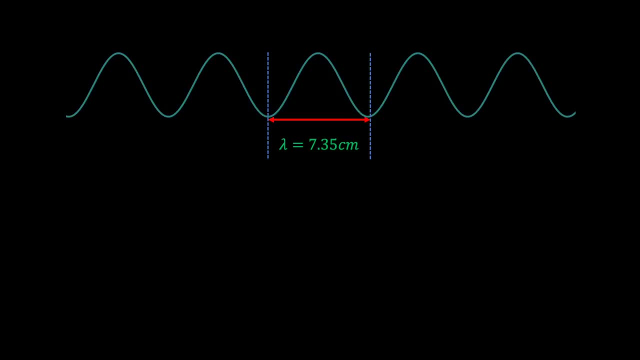 antenna output, the result would be equal to zero within the bounds of experimental uncertainty. However, when Penzias and Wilson began taking measurements in the spring of 1964, they were surprised to find a very strong signal of microwave noise at 7.35 centimeters. 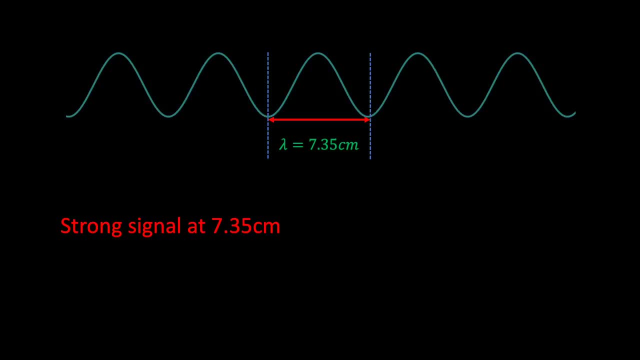 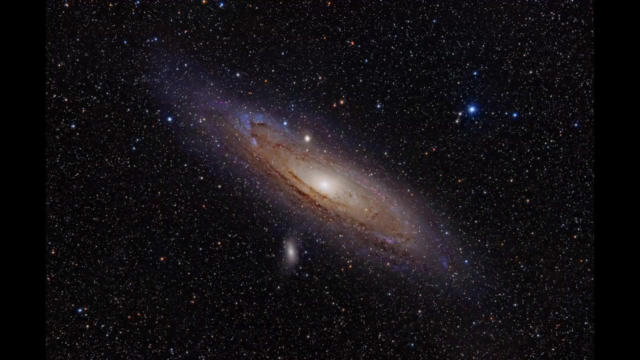 What was even more perplexing was that the strength of the signal appeared to be independent of the direction they pointed the antenna, as well as the time of day or the season. Furthermore, Penzias and Wilson realized that the signal could not be coming from our own galaxy, because if it was, then you would expect. 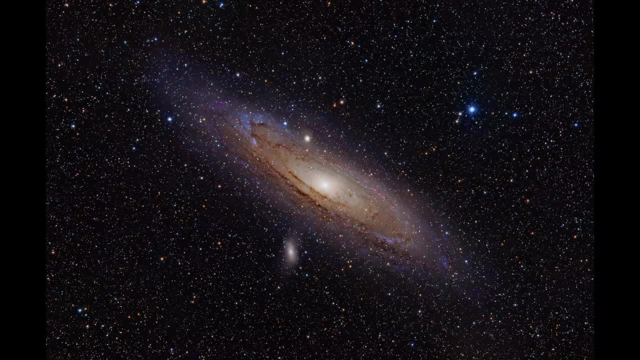 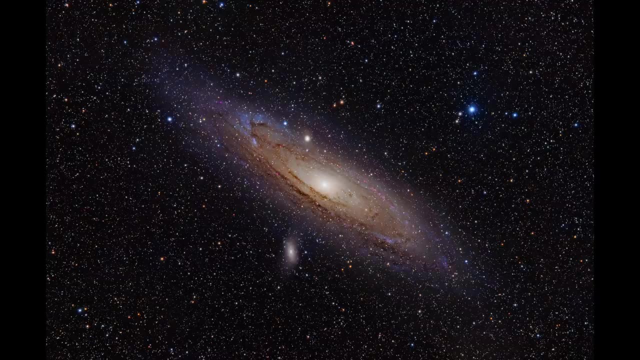 to see a similar strong signal originating from other galaxies, like our nearest neighbor, Andromeda. However, no such signal had been detected. This lack of dependence on direction suggested that in your own galaxy there was a that the microwave noise was coming from a much larger volume of the universe than just our own. 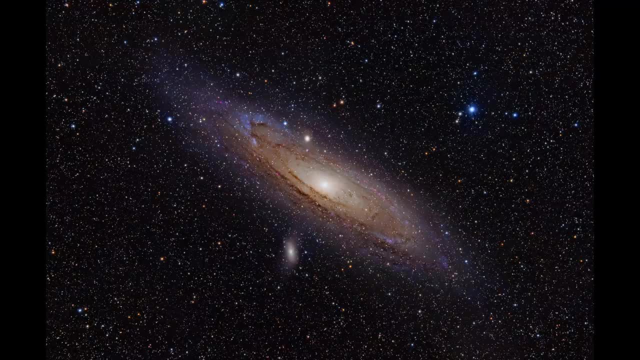 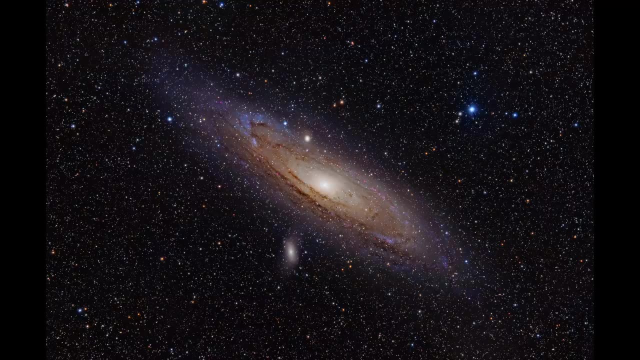 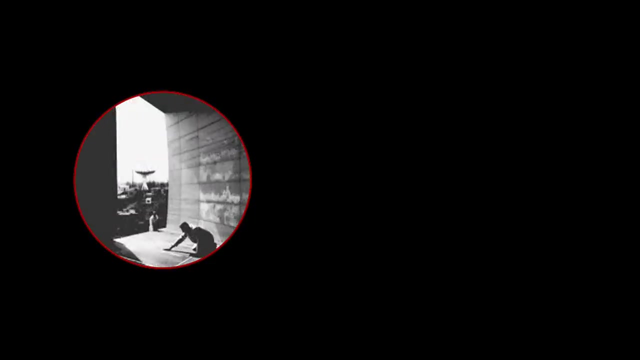 galaxy. However, Penzias and Wilson could not shake the idea that perhaps this radiation was simply antenna noise and they had somehow missed or failed to identify its source. They were so convinced by the idea that there must be some kind of antenna noise that they took apart the apparatus and 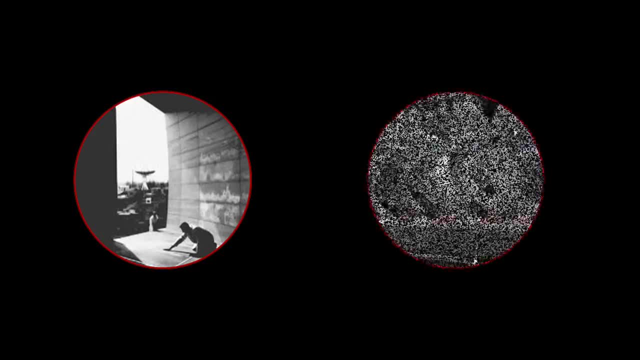 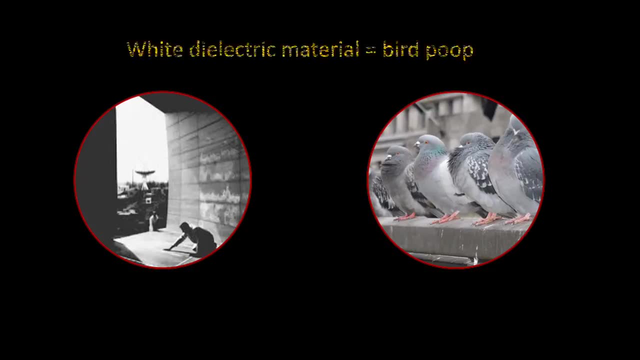 thoroughly cleaned it, Not least of all because they had found a pair of pigeons had been roosting in the throat of the antenna and had covered the surface in what Penzias delicately described as a white dielectric material which could, at room temperature, be a source of electrical noise. 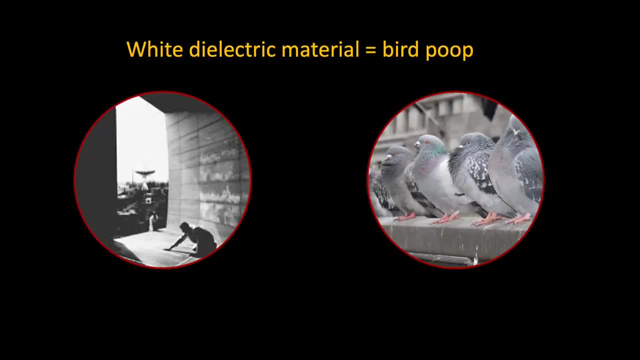 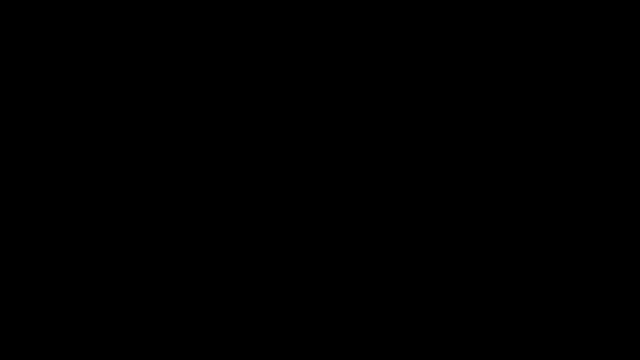 However, after dismantling, cleaning and rebuilding the antenna, the mysterious noise was still there, undiminished. So what was this microwave noise and where was it coming from? Although Penzias and Wilson had no idea where the radiation was coming from, the one piece of numerical data that they 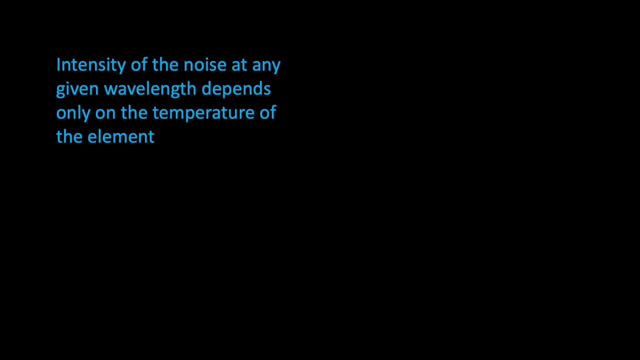 did have was that it was coming from a microwave. So what was this microwave noise and where was it coming from? So what they did have was the intensity of the microwave noise. Penzias and Wilson knew that any electrical circuit element at a temperature above absolute zero generates noise as a consequence of. 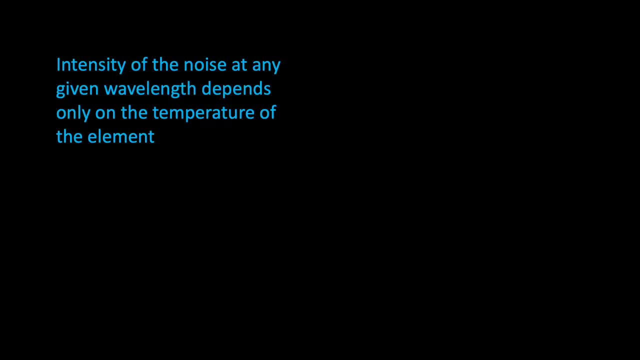 the thermal motion of electrons. Furthermore, the intensity of the noise at any given wavelength depends only on the temperature of the element. The hotter the element, the more intense the noise. Penzias and Wilson realised that they could use this relationship in reverse to assign an effective 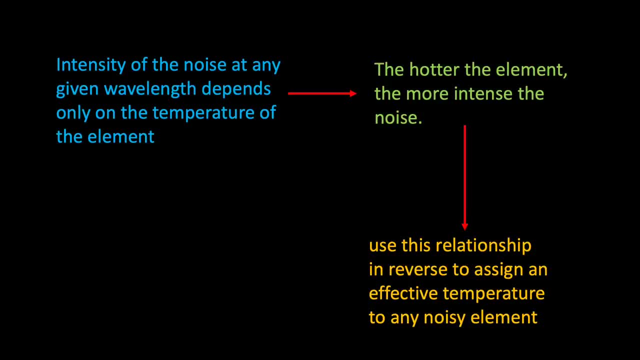 temperature to any of the elements. So what was this microwave noise and where was it coming from? So what was this microwave noise and where was it coming from, Regardless of whether the noise is of thermal origin or not? Using this technique, Penzias and Wilson found that the effective temperature for their observed 7.35. 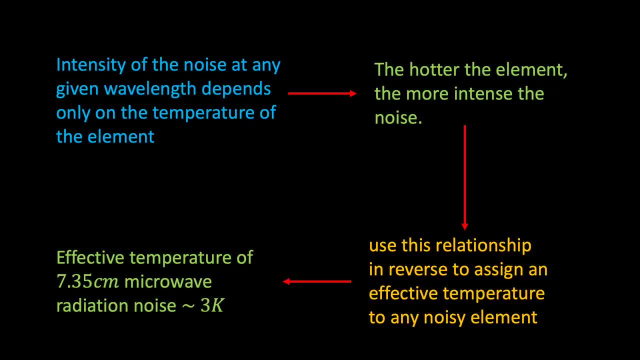 centimetre microwave radiation noise was around three degrees above absolute zero or three kelvin. This was much greater than expected, but very low in absolute terms. Penzias and Wilson remained thoroughly puzzled by the situation, but they were determined to track down the source of the. 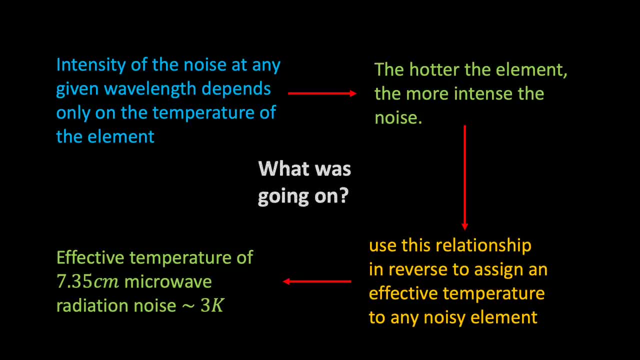 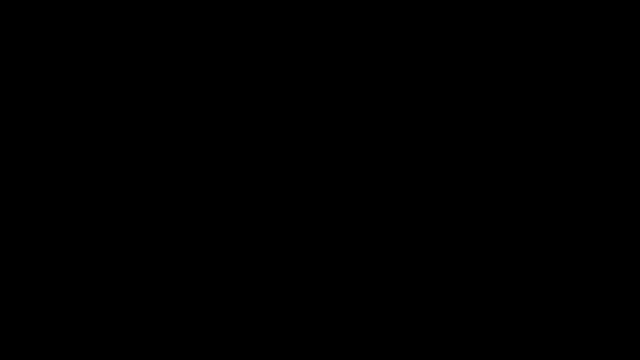 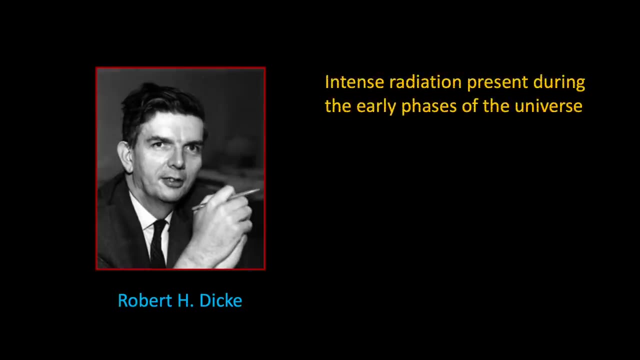 enigmatic signal. So what was this microwave radiation? What was going on? A possible explanation for the mysterious microwave radiation was put forward by a small group of theorists at Princeton, spearheaded by Robert Dickey. Dickey had suggested that there must have been an intense background of radiation present during the first few minutes of the 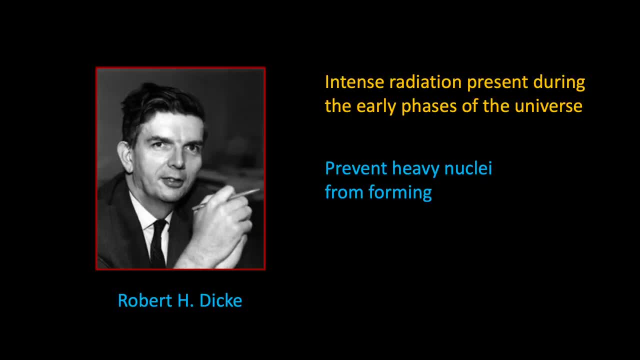 universe. otherwise, it would have been possible for nuclear reactions to proceed so rapidly that most of the hydrogen would have been fused to form heavier elements. This is in direct contradiction with what we actually observe in the universe where we see. roughly three quarters of visible matter is comprised of hydrogen. 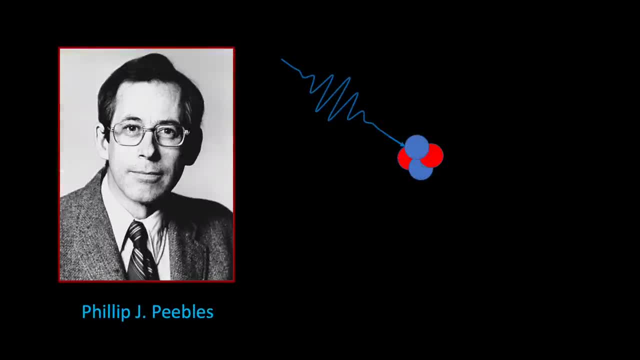 Following Dickey's suggestion, a young theorist named Jim Peebles enthusiastically calculated the consequences of a hot early phase in the history of our universe and demonstrated that rapid fusion could have been prevented if the early universe had been bathed with intense radiation at extreme temperatures and temperatures. This is in direct contradiction with what we actually 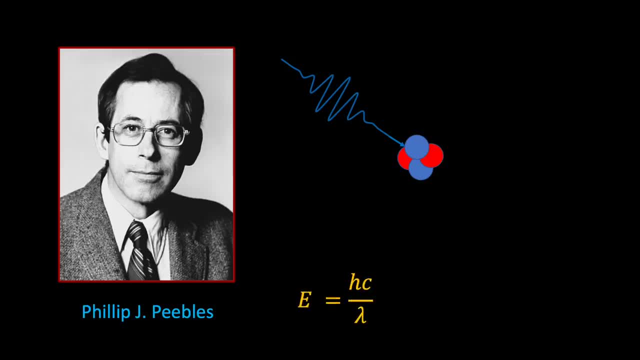 observe in the universe where we see, roughly three quarters of visible matter is comprised of hydrogen. very short wavelength. according to einstein's famous photon energy relationship, the shorter the wavelength, the higher the energy. if the photon energy was high enough, it would have been possible. 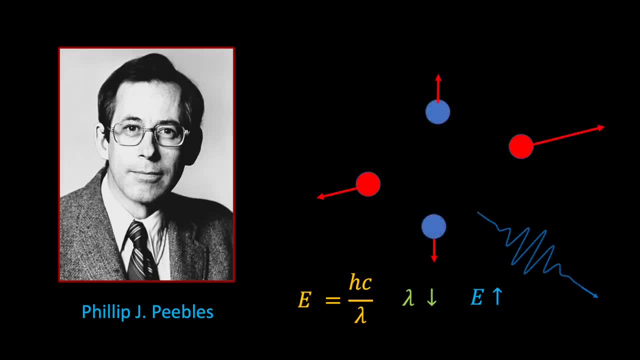 to break apart any nuclei that formed. furthermore, people's was also able to show that the subsequent expansion of the universe would have caused the wavelength of the radiation to increase and therefore cause the equivalent temperature to reduce significantly. people's estimated that in all order for the background radiation to have kept the production of helium and heavier elements in 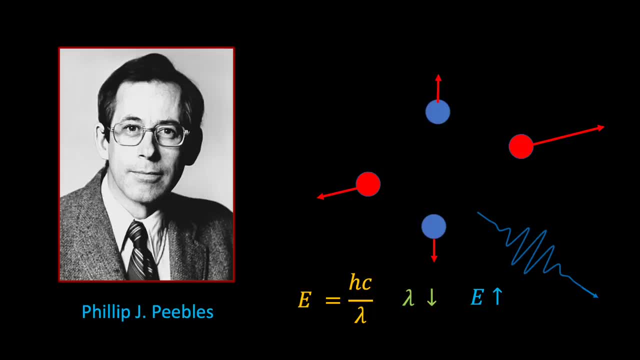 check and within known bounds, it would have had to be so intense that its equivalent temperature today would be close to the value measured by penzias and wilson. this was remarkable. if people's calculation was correct, then the background microwave radiation detected by penzias and wilson 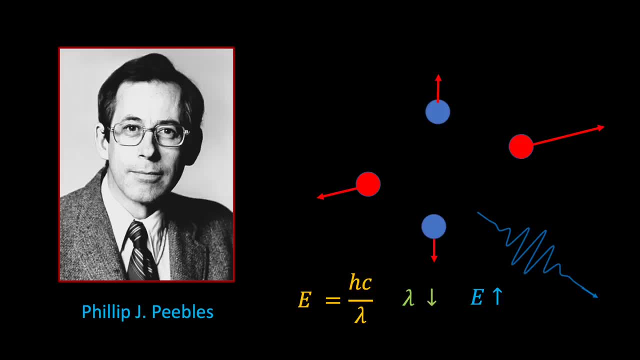 was in fact the afterglow of the big bang, so was people's correct? is the microwave radiation actually left over from the beginning of the universe? to answer this question, we will need to delve into a little bit of theory. what are the general properties of the radiation that should be? 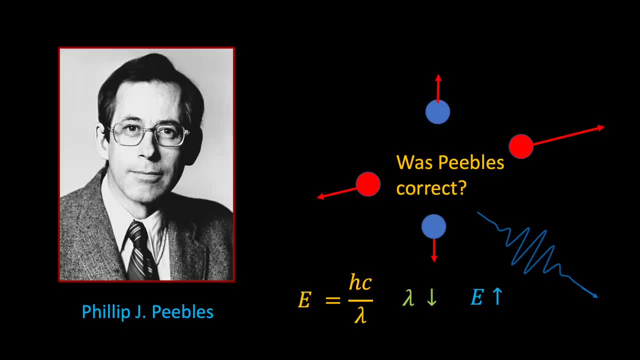 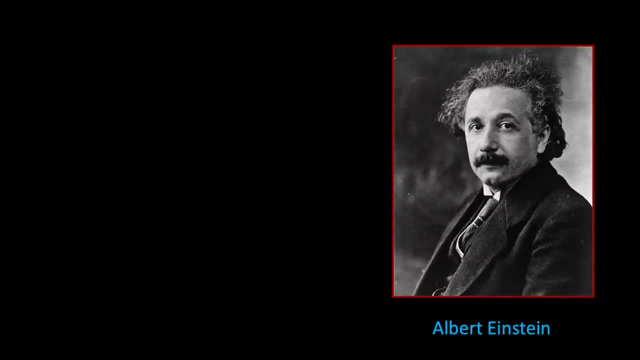 filling the universe, if current cosmological ideas are correct. and what happens to this radiation as the universe expands? firstly, we need to give up the classical picture of radiation in terms of electromagnetic waves and switch to the quantum view that radiation consists of particles known as photons, as put forward by 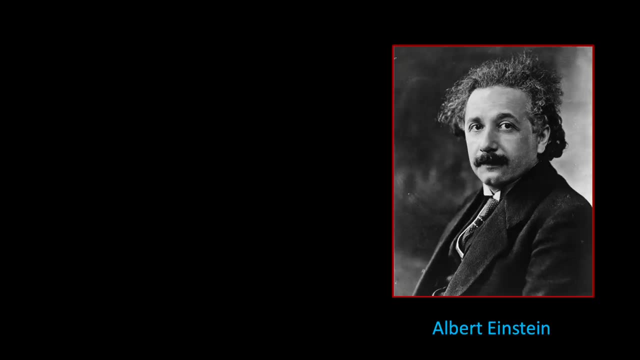 einstein in 1905. an everyday light wave contains an enormous number of photons traveling along together. classically, the energy is assumed to be continuous. if, however, we were to measure the energy of a light wave with extreme precision, we would find that it always comes in multiples of a. 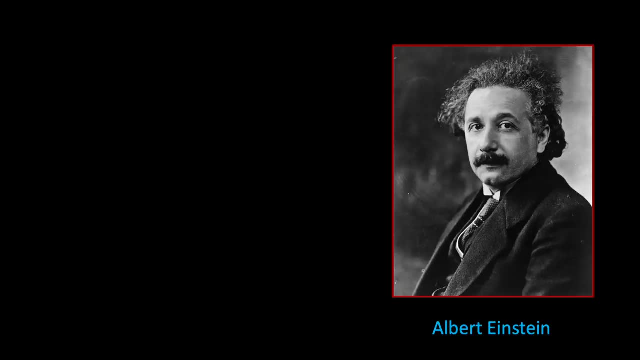 discrete amount of energy equal to the energy of a single photon. if f is the frequency of the light wave, then each photon will have an energy equal to hf or hc over lambda, where lambda is the wavelength, and the total energy of the wave will be equal to n times the photon energy. 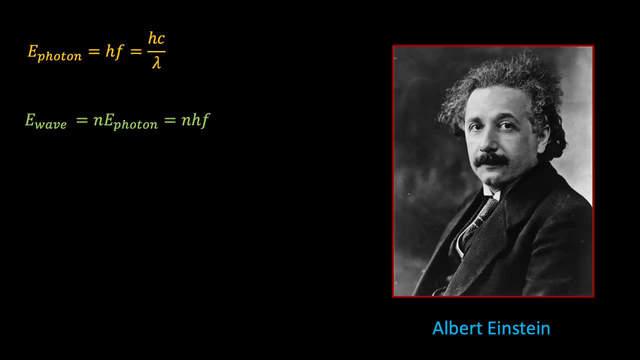 where n is the number of photons. to give you an idea of typical photon energies, visible light emitted from the surface of the sun has a peak wavelength of around 550 nanometers and therefore we see that the energy of a single photon of this wavelength will be around 3.6 times 10 to the. 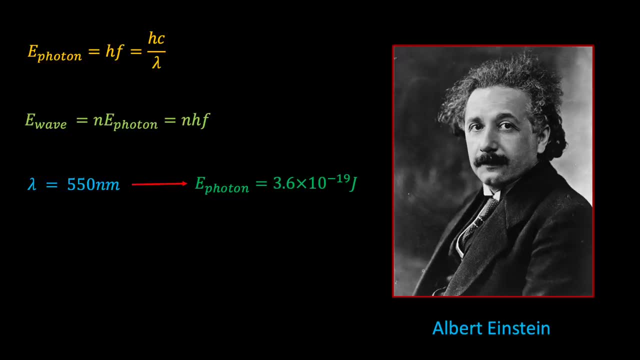 minus 19 joules. when dealing with such small energies, it's often convenient to rewrite the energy in terms of electron volts, where one electron volt is defined as the energy transferred to an electron when it moves through a potential difference of one volt, in other words, one electron. 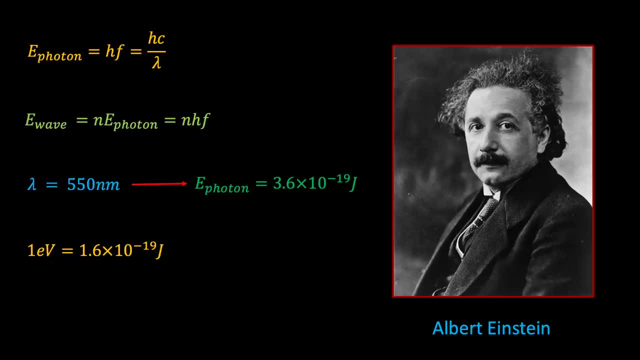 volt is equal to 1.6 times 10, to the minus 19 joules, and therefore, if we write our photon energy in terms of electron volts, we see that the photon energy is 2.26 electron volts. by way of comparison, consider a hydrogen atom comprising one proton and one electron. 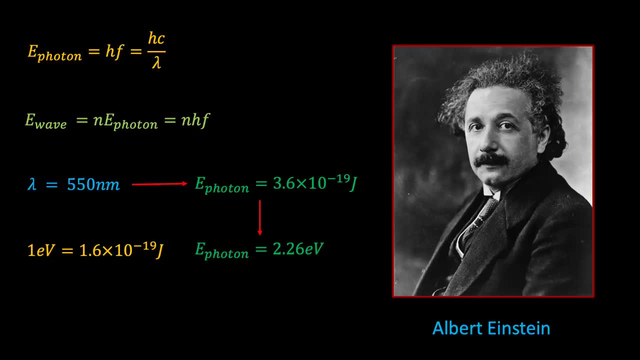 the proton and electron are held together by the electrostatic force of attraction acting between them. however, if the electron inside the hydrogen atom is given sufficient energy, it can be ripped out of the atom in a process called ionization. the ionization energy of a hydrogen atom is 13.6. 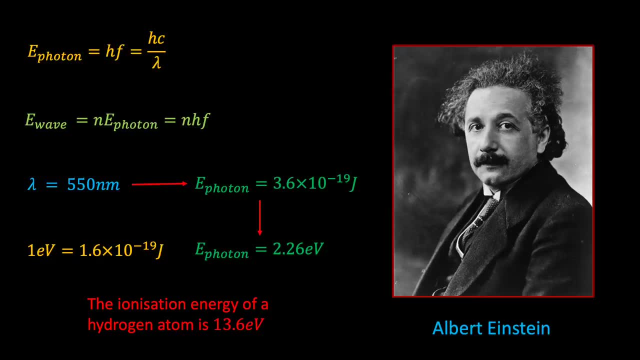 electron volts. so what might cause ionization to occur? well, one way would be for an electron to absorb a high energy photon which has sufficient energy to kick the atom electron out of the atom. and, as we have seen, the energy of a single photon is determined by the 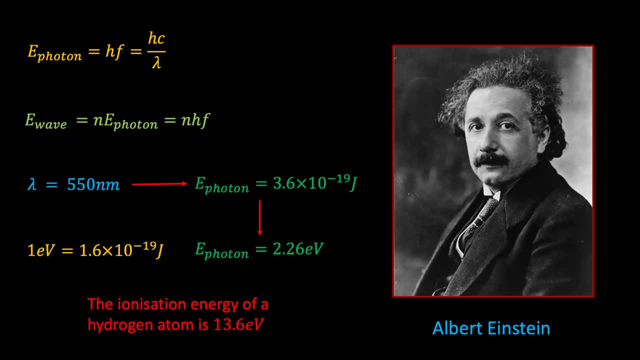 wavelength of the light, we see that photons comprising visible light do not have sufficient energy to do this. however, if a gas cloud of hydrogen was bathed in high frequency, short wavelength light, then the photons comprising the light would have enough energy to ionize the hydrogen and stable hydrogen atoms would be unable to form. keep this in mind as we consider the 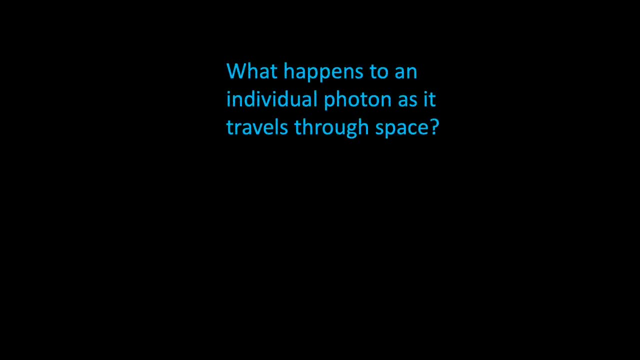 following question: what happens to an individual photon as it travels through the universe? well, it turns out not much, since most of the universe is empty space. using modern day telescopes, we're able to see objects over 10 billion light years away, implying that the light has managed to travel unimpeded for 10 billion years across the vast reaches of space. this 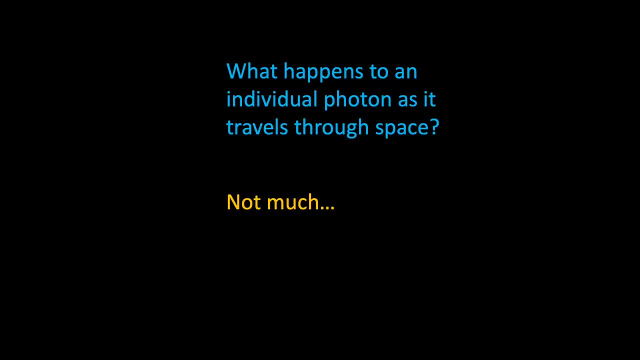 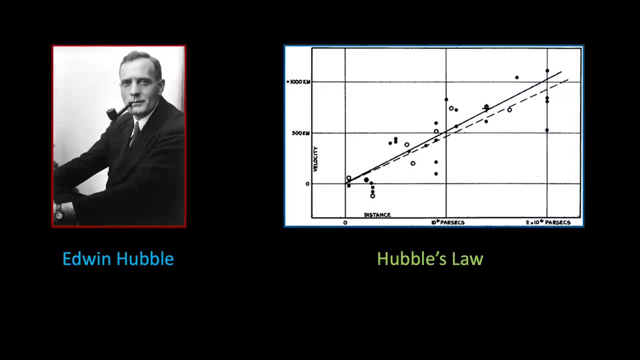 indicates that whatever matter may be present in the universe, it is sufficiently transparent so that photons can travel for very large distances without being scattered or absorbed. however, this was not always the case. the work of edwin hubbell in the 1920s revealed that the light from distant 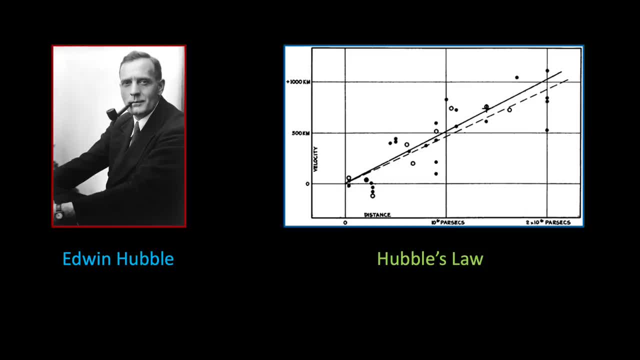 galaxies was red shifted, meaning that the universe is expanding and therefore its contents must have been squeezed into a smaller region in the past. now it's well known that the temperature of a fluid will generally rise when the fluid is compressed, and therefore we expect that the universe will be able to travel for very large distances without being scattered or absorbed. 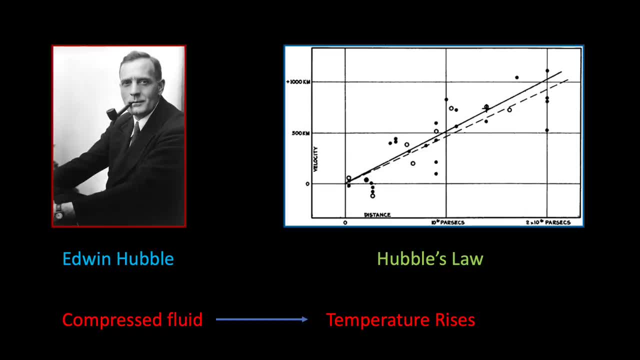 in fact, there would have been a time when the contents of the universe was so hot that it would have been impossible for electrons and protons to combine to form stable atoms, since the average energy of the electrons would have exceeded the ionization energy of hydrogen, meaning that the protons were unable to catch hold of the electrons to form stable hydrogen atoms. 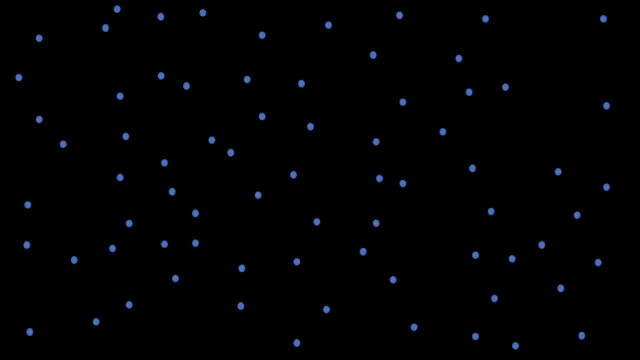 under these extreme conditions, an individual photon would not have been able to travel for far without being scattered or absorbed by an electrically charged nuclear electron. the average time between photon interactions with matter was extremely short, and even though the universe was expanding very rapidly at first, from the perspective of an individual photon or electron, 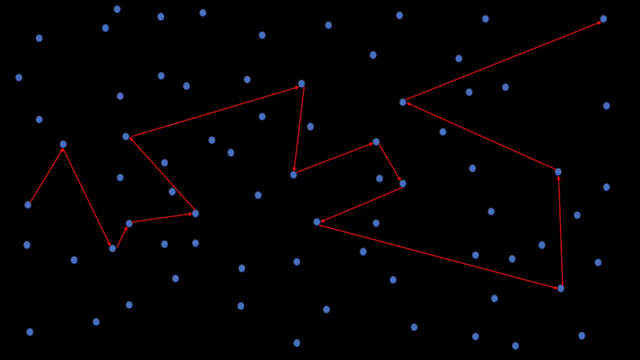 or nucleus. the expansion was slow enough for each photon to be scattered or absorbed and re-admitted many times as the universe expanded. now, any system in which the individual constituents have time to interact multiple times, usually in the form of a single electron, is the time to interact with the. 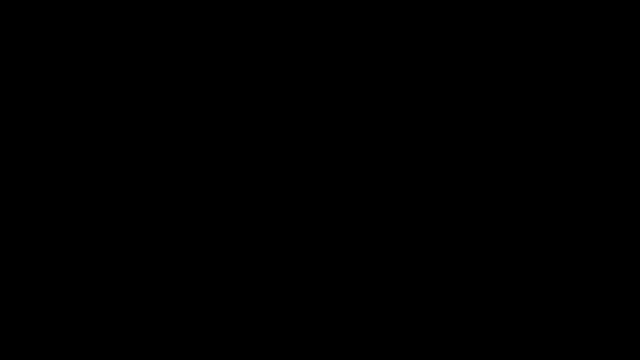 electron in the form of a single electron. in the form of a single electron in the form of a single electron. so what is equilibrium? well, although the individual speeds and energies of the constituent particles may be changing, the overall statistical distributions of those speeds and energies would remain constant. equilibrium of this kind is often called thermal equilibrium, because it is. 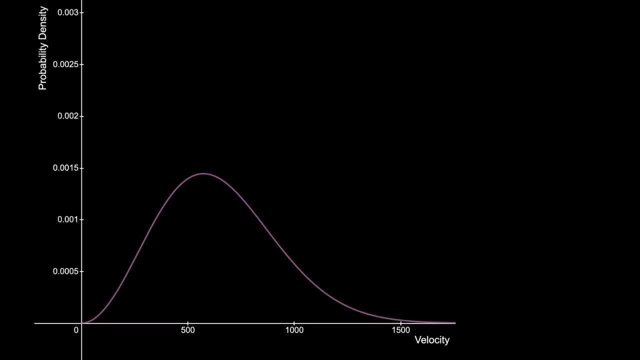 characterized by a definite temperature which is essentially the same throughout the system. now it turns out that the properties of any system in thermal equilibrium are entirely determined once we specify the temperature of the system and the densities of a few conserved quantities. furthermore, we have seen that, according to peebles, the cosmic microwave 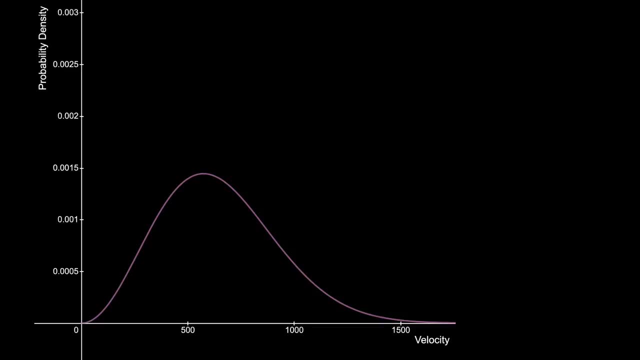 radiation discovered by penzias and wilson is believed to have originated from the early stages of the universe, at a time when, as we have just argued, the universe was in a state of thermal equilibrium. therefore, in order to properly understand the characteristic features of the cosmic microwave radiation, 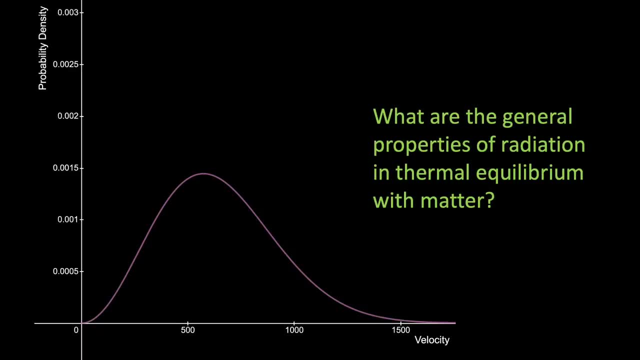 we need to understand the general properties of radiation in thermal equilibrium with matter, and therefore it is worthwhile taking a short detour to understand the radiation properties of hot objects. by the 1890s it was known that the properties of radiation in a state of thermal 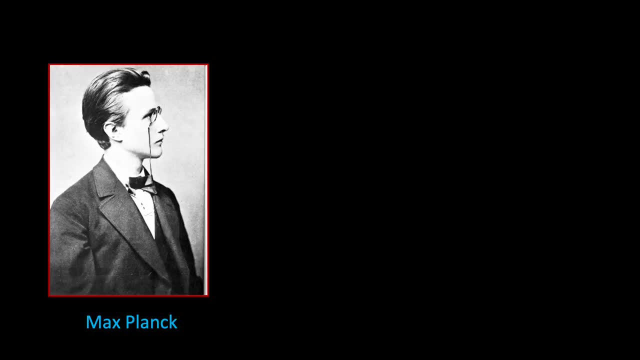 equilibrium with matter depend only on the temperature. it became a question of vital importance to understand and explain how the intensity of radiation emitted by a hot object varied with temperature and wavelength. in this case, the energy of the hot object was limited to a particle with a temperature higher. 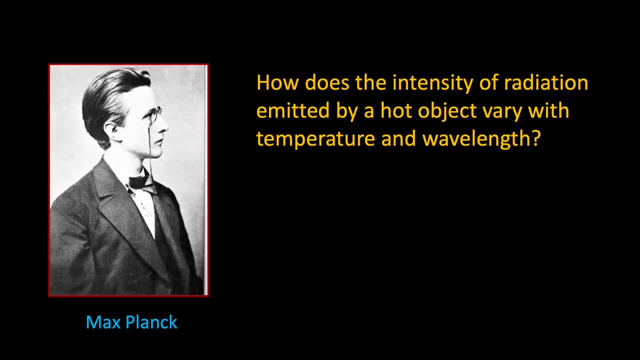 than zero. at the time, the best known laws of classical physics were unable to provide an adequate explanation. in fact, the situation was even worse. the best known laws of classical physics predicted that any object with a temperature above absolute zero should be emitting an infinite amount of high frequency radiation. because high frequency radiation was. 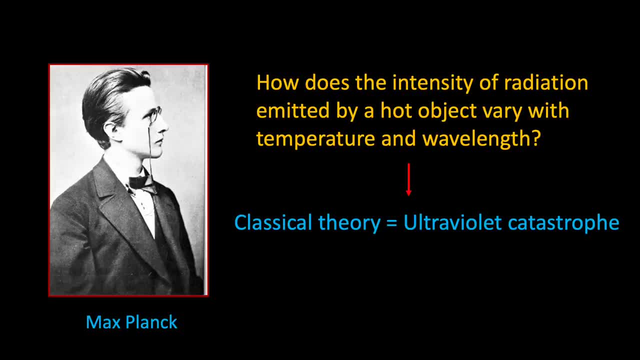 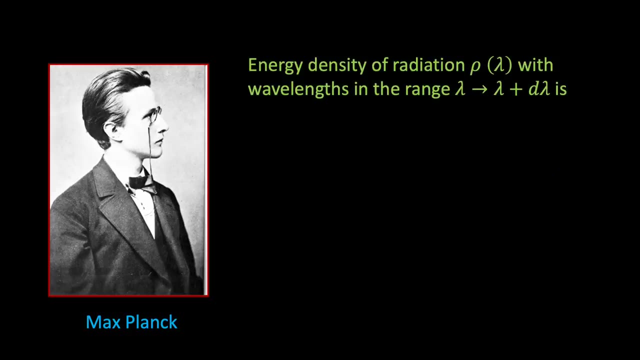 dubbed ultraviolet radiation. this problem became known as the ultraviolet catastrophe, famously forced to introduce the concept of energy quantization at the beginning of the 20th century. Planck's famous radiation law states that the energy density of radiation with wavelengths in the range lambda to lambda plus d lambda is given by the following yellow expression: 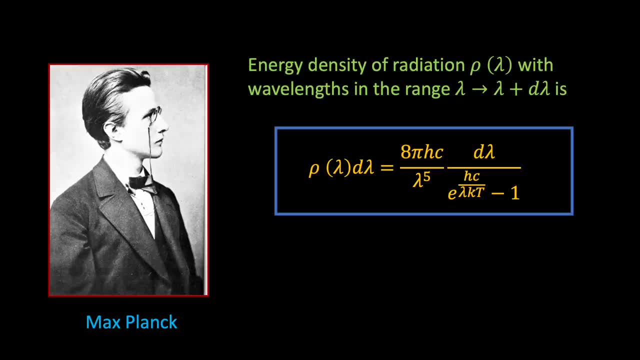 where lambda is the wavelength, c is the speed of light, h is Planck's constant, k is the Boltzmann constant and t is the temperature in kelvin. Now, this may look like a slightly intimidating mathematical expression, so let's instead visualize this function by plotting a graph. 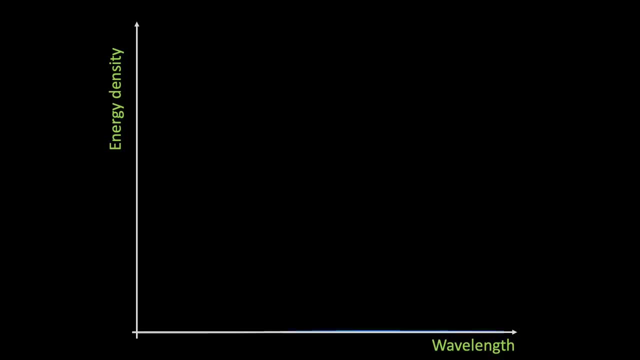 If we plot a graph with wavelength on the x-axis and energy density on the y-axis and then slowly increase the temperature from zero, we see that as the temperature increases, the wavelength corresponding to peak energy density decreases. This is familiar from everyday experience If you put a bar of metal in a hot fire, as the temperature of the metal increases, 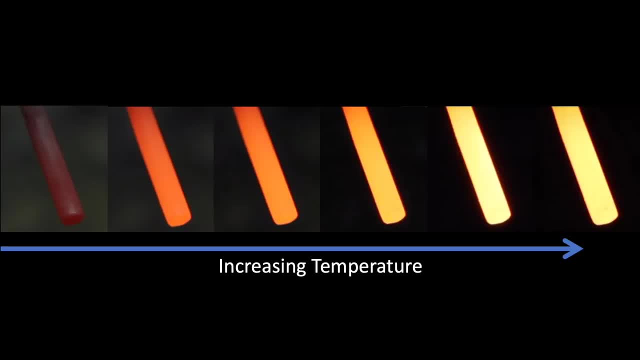 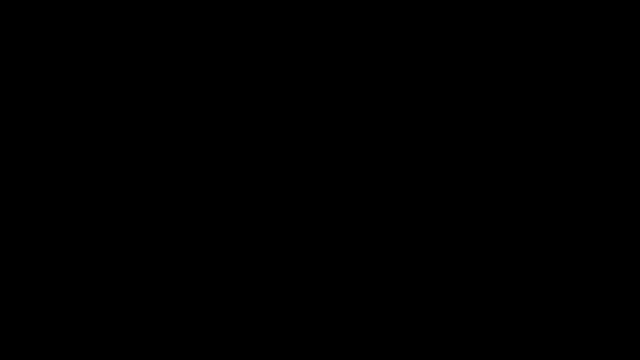 it will first start glowing: dull red, then orange, and then blue, Then orangey red, then bright yellow and finally intense bluey white light as the temperature increases. And so we see from Planck's radiation law that the wavelength of the most intense light 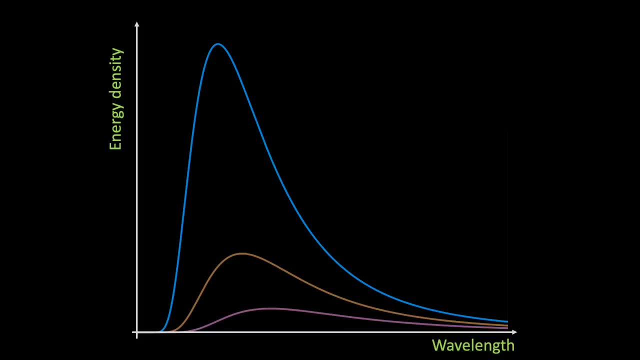 emitted from the object decreases with temperature. Furthermore, we see that the area under the curve, which corresponds to the total energy density of radiation, increases with temperature. In other words, hotter objects emit more light than cooler objects. So a natural question of: 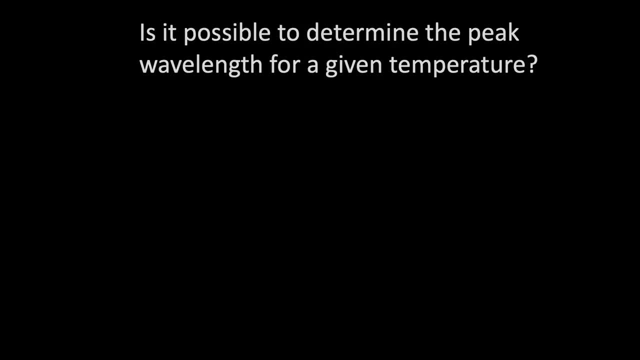 course arises. is it possible to determine the peak wavelength of the emitted radiation for a given temperature? Well, the answer is yes, and because this result is going to prove crucial in unlocking the mystery of the microwave radiation, it's worth spending a few moments. 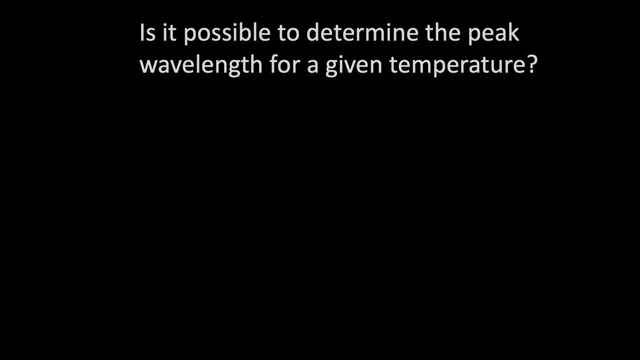 delving a little deeper. Firstly, in order to find the maximum value of Planck's radiation function, we simply need to differentiate the energy density expression and set it equal to zero. In order to differentiate this expression, we need to make use of the well-known product rule. If we apply this to the Planck, 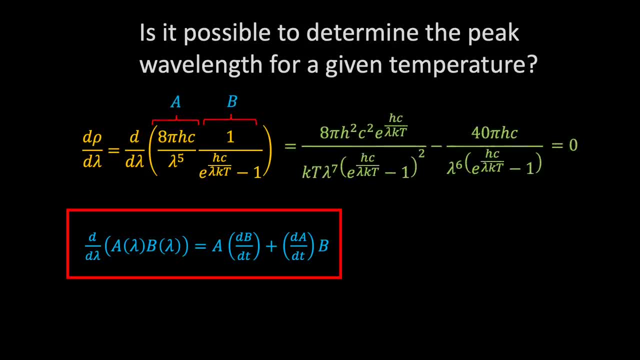 law expression and simplify the algebra, we find the following ghastly green expression: Next, if we let x equal hc over lambda kt, then after a bit of rearranging and simplifying you should be able to convince yourself that the condition d rho by d lambda equals zero. 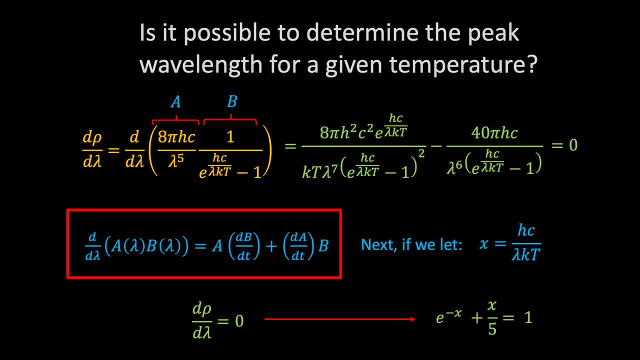 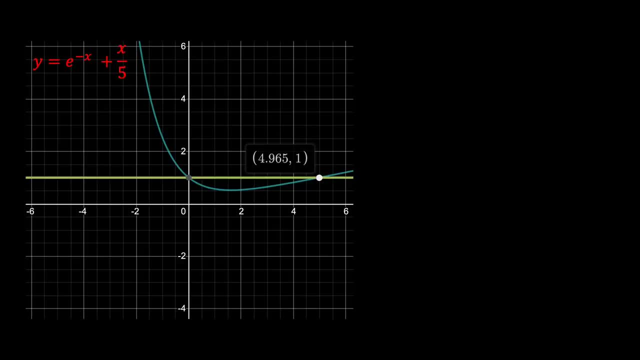 can be written as: e to the minus x plus x over five equals one. Now this equation can be used to find the maximum value of radiation, and it can be solved graphically by plotting: y equals e to the minus x, plus x over five and y equals one, and observing where the lines intersect, We see from the graph that they 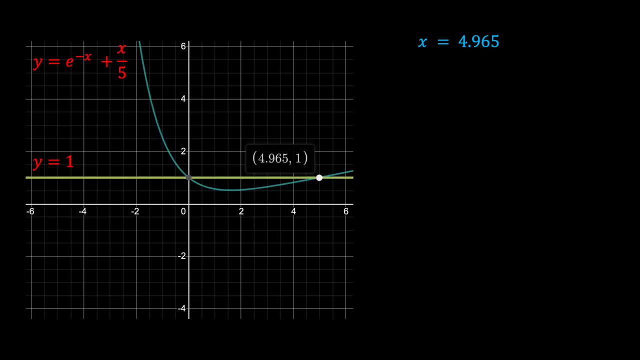 intersect at a value of x equals 4.965, and therefore we can write hc over lambda kt equals 4.965.. And if we rearrange for lambda t, we find the following relationship: If we plug in the values for Planck's constant and the speed of light and simplify, we finally: 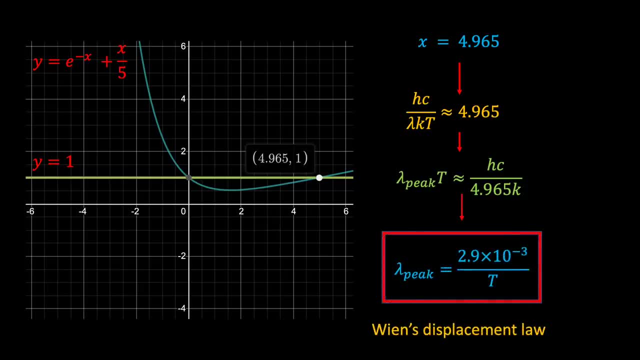 arrive at a very famous equation known as the Wien's displacement law. Wien's displacement law states that the radiation curve for different temperatures will peak at different wavelengths that are inversely proportional to the temperature. Now we can see from Wien's law that at a temperature 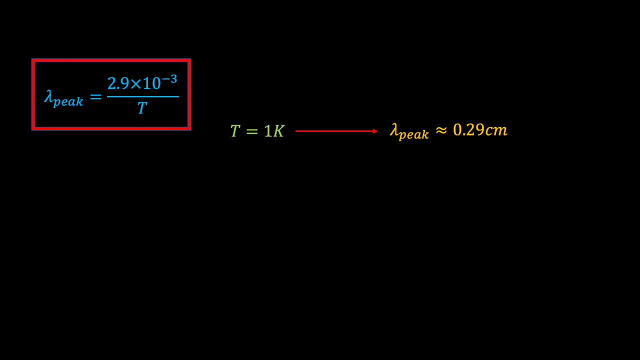 of one kelvin. peak emission will occur at a wavelength of 0.29 cm, which is in the microwave wavelength region of the electromagnetic spectrum, whereas an opaque body at a room temperature of 10 micrometres will emit infrared radiation with a wavelength of 10 micrometres, which is about 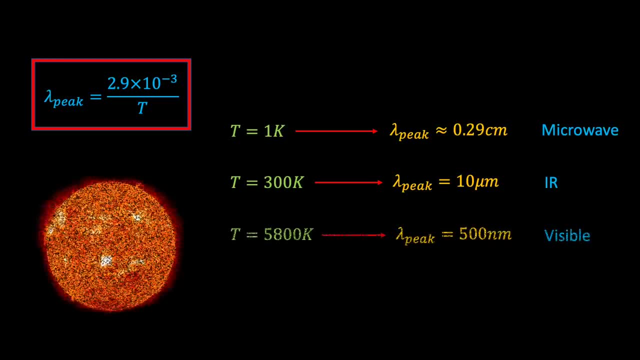 a thousandth of a centimetre. On the other hand, the surface of the sun is at a temperature of 5,800 kelvin and consequently emits visible light at a wavelength of around 500 nanometres. The fact that the wavelength of visible light is so small helps explain why the wave nature of light. 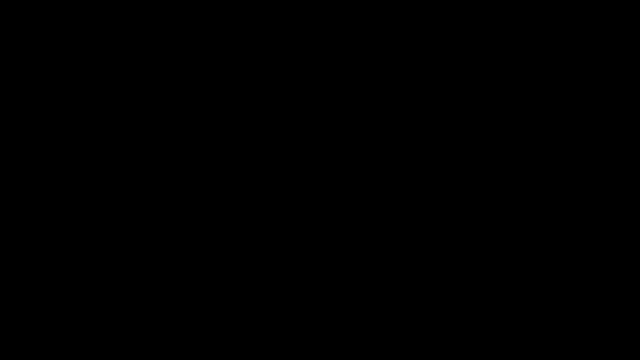 took so long to discover. Okay, so the Wien's displacement law tells us the peak wavelength, but what if we want to determine the total energy density of the emitted radiation for all wavelengths at a given temperature? Well, in that case we simply need to integrate the Planck radiation. 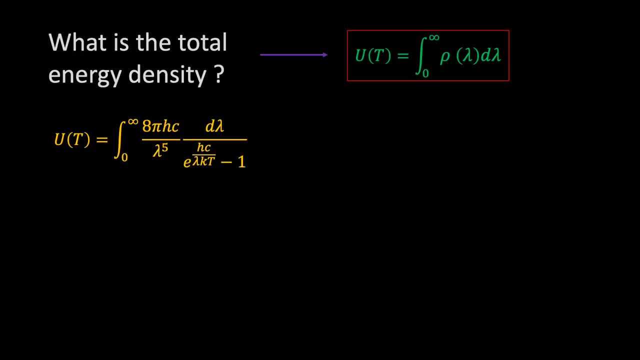 expression with respect to wavelength from zero to infinity. To make life easier, let's again define: x equals hc over lambda kt, in which case it follows that d lambda can be written as the following blue expression: and so if we replace lambda and d lambda, we find the following yellow: 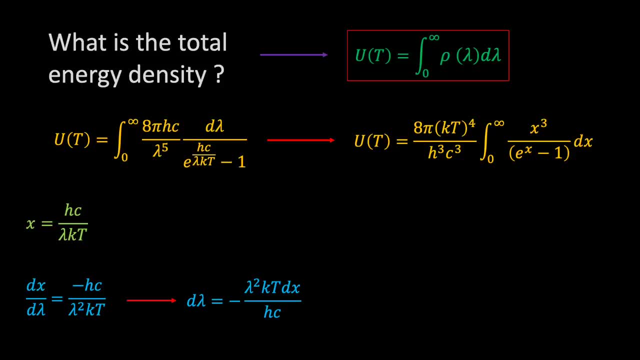 expression. Now, the good news is that the integral of x, cubed over e to the x minus 1, is a standard integral, which is equal to pi to the 4 over 15, and so if we put everything together, we find the following light blue expression: This is known as the Stefan-Boltzmann law, and it relates the energy. 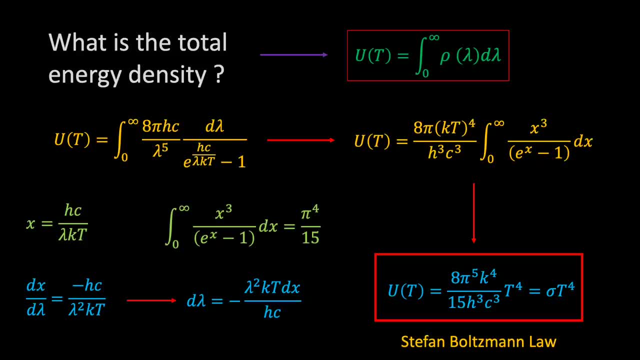 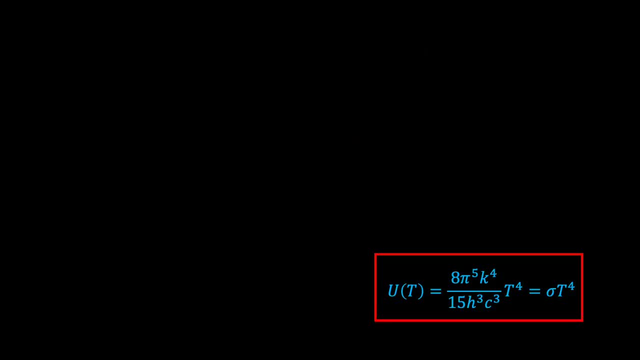 density of a hot object to the temperature of the object. More specifically, we see that the energy density is proportional to the fourth power of the temperature. To put this in concrete terms, let's use the Stefan-Boltzmann law to calculate the energy density at a temperature of 1 kelvin. 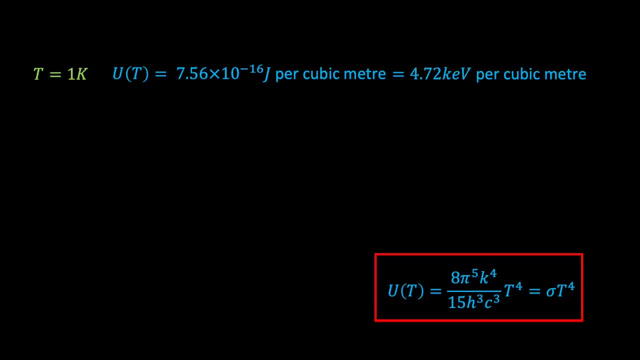 in which case we find a value of 4.72 kiloelectron volts per cubic meter. Now if the cosmic microwave background radiation discovered by Penzias and Wilson really is thermal radiation at a temperature of around 3 kelvin, then its energy density will be 383 kiloelectron volts per meter cubed. 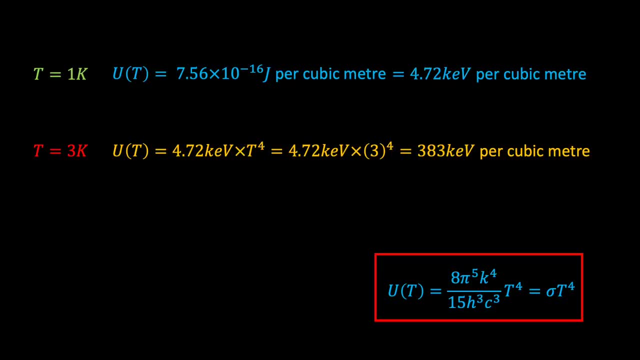 and it's worth noting at this stage that if the temperature is a thousand times higher than that at 3000 kelvin, the energy density will be a trillion times higher. In other words, the energy density would be 3.83 times 10 to the power of 14 kiloelectron volts per meter cubed. 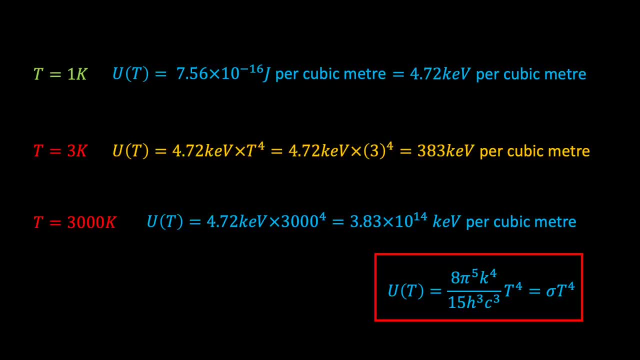 Ok, so the Stefan-Boltzmann law allows us to determine the energy density at a given temperature, but what has this got to do with the cosmic microwave background radiation of Penzias and Wilson? Well, as we've already seen, there must have been a time during the early universe when 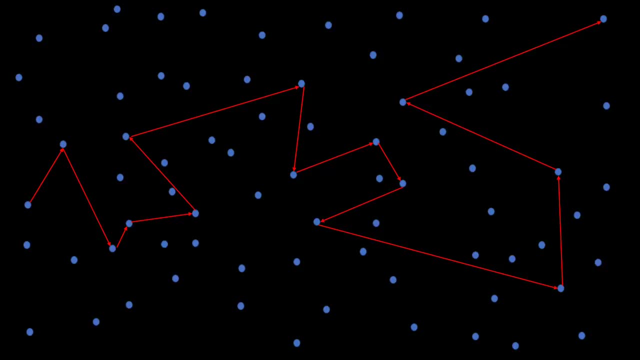 photons were so high that atoms were dissociated into their nuclei and electrons, and the scattering of photons by free electrons maintained a thermal equilibrium between matter and radiation. As time passed, the universe expanded and cooled, eventually reaching a temperature which was low enough to allow the combination of nuclei and electrons into atoms. The sudden disappearance. 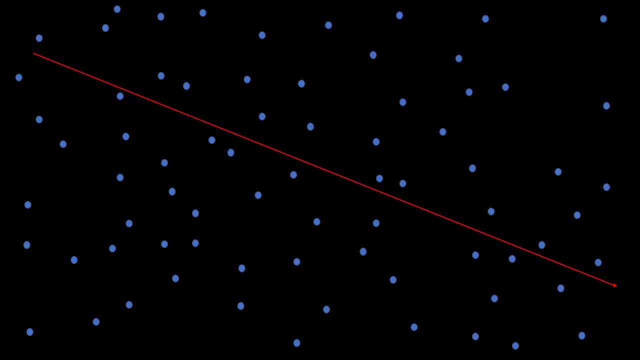 of the free electrons allowed the photons to travel greater distances without being absorbed or scattered, and thus the thermal contact between the atoms and the electrons was reduced. The radiation continued to expand freely. In cosmology, this moment is referred to as recombination, the epoch when charged electrons first became bound to protons to form atoms. 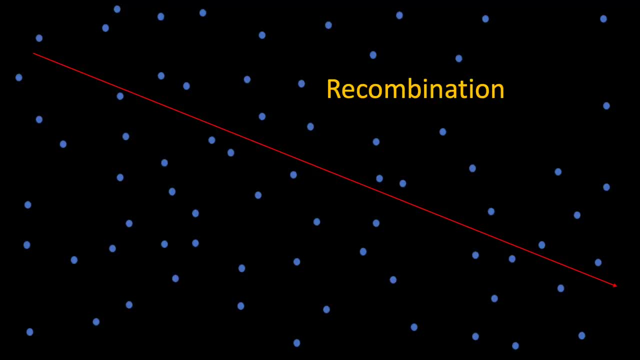 Now, the term is a little misleading, as it implies that the protons and electrons prior to this moment were once bound, though this is certainly not true according to the Big Bang theory, since the temperature in the earliest phases of the universe would have been: 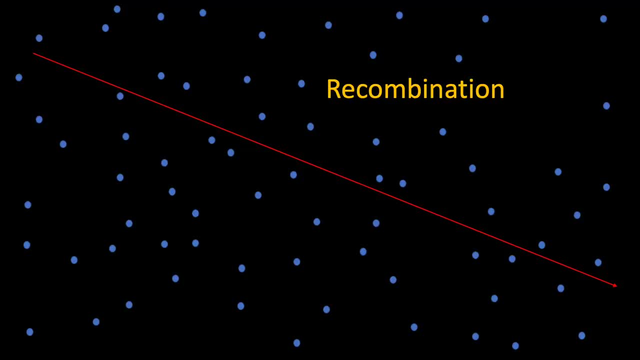 too high. The temperature in the earliest phases of the universe would have been too high. The important point here is that at this moment of recombination the Steffen-Boltzmann law tells us the total energy density of the radiation at all wavelengths and says it would have been. 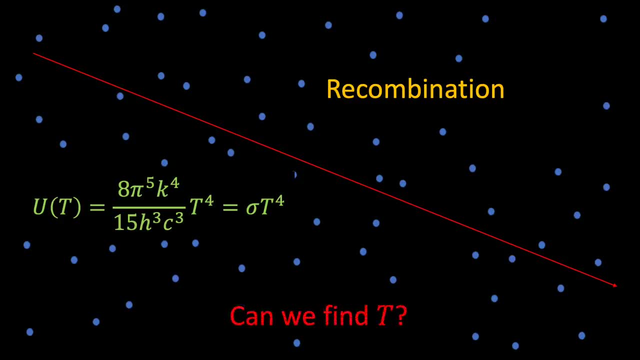 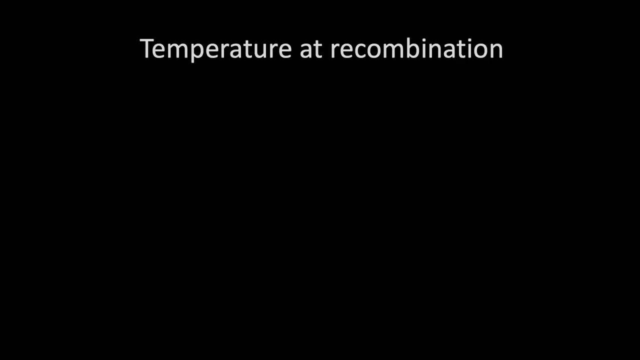 determined by the fourth power of the temperature. So we can certainly estimate the temperature. Recall that the Planck distribution can be interpreted in terms of photons. Each photon has energy hc over lambda, hence the number of photons dn per unit volume in a narrow 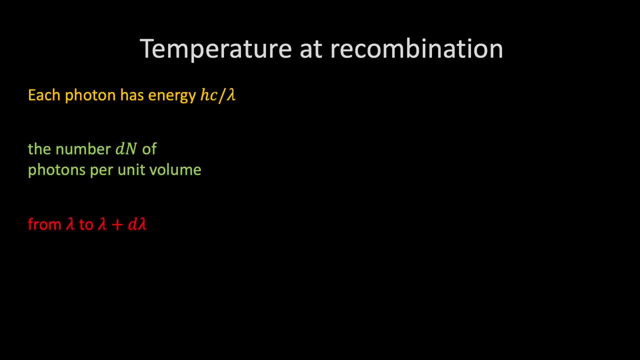 range of wavelengths from lambda to lambda plus d lambda is given by the energy density divided by the energy of a single photon. If we want to find the number density for all wavelengths, we need to integrate over all wavelengths, from zero to infinity. This is a standard integral involving 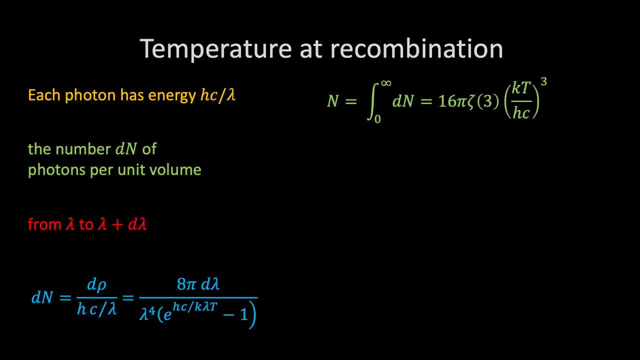 the Riemann zeta function, which I suggest you check using Wolfram alpha. If we then sub in the values of Boltzmann's constant, Planck's constant and the speed of light, we find that the number of photons per cubic centimeter is roughly 20.28 times the cube of the temperature. 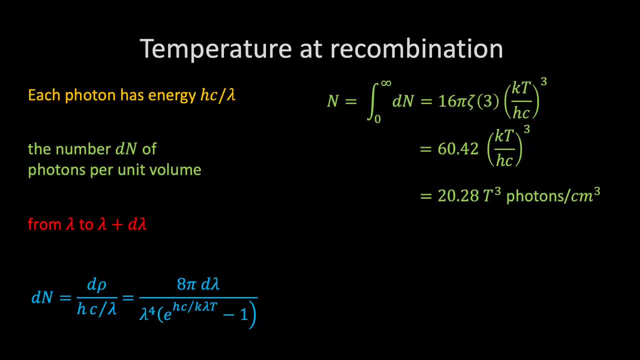 We can then combine this result with the Stefan-Boltzmann law to calculate the average photon energy, as this will simply be the total energy density divided by the number density, and we find a value of 3.73 times 10 to the minus 23 times the temperature T. So we see: 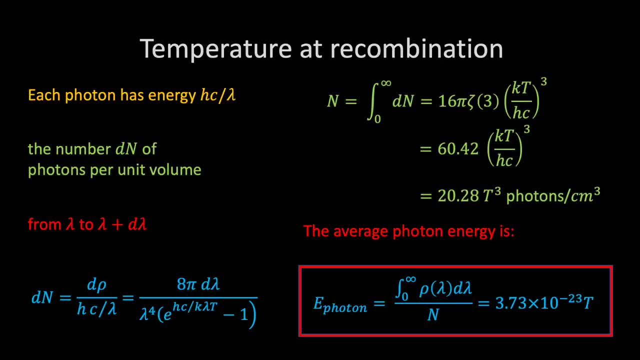 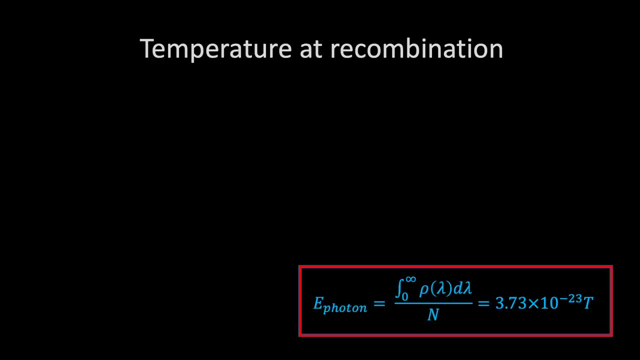 that the average photon energy is directly proportional to the temperature. Now that we have an expression for the average photon energy at a given temperature, we can estimate the temperature at which recombination occurs. To do this, we will set the average photon energy equal to the ionization energy of hydrogen, as this represents the energy needed to remove the 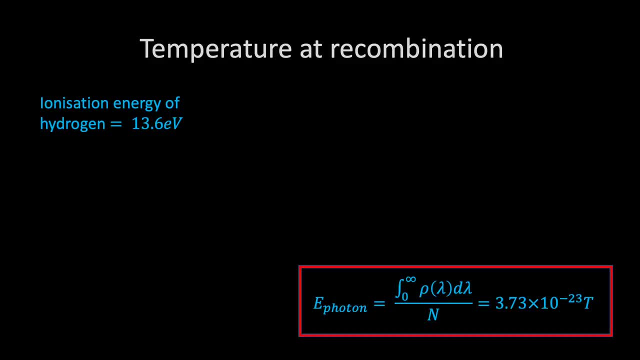 electron from the proton inside a hydrogen atom. We saw earlier that the ionization energy of hydrogen is 13.6 electron volts, and so we see that by rearranging the expression for the average photon energy, we arrive at an estimated recombination temperature of around 60 000 kelvin. Now it's 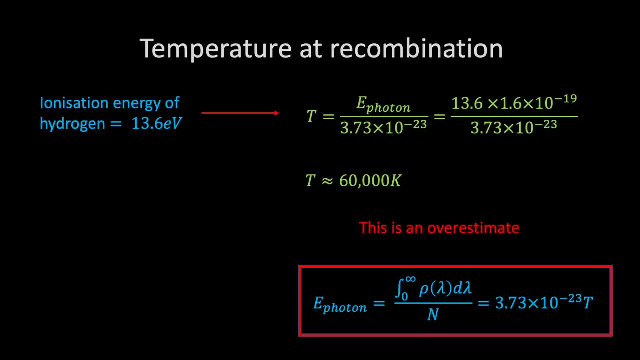 very important to emphasize that this is an overestimate for the temperature of recombination. But why? Well, this has to do with the relative number density of photons compared to protons and neutrons in the universe. Experimental data suggests there are roughly one billion photons. 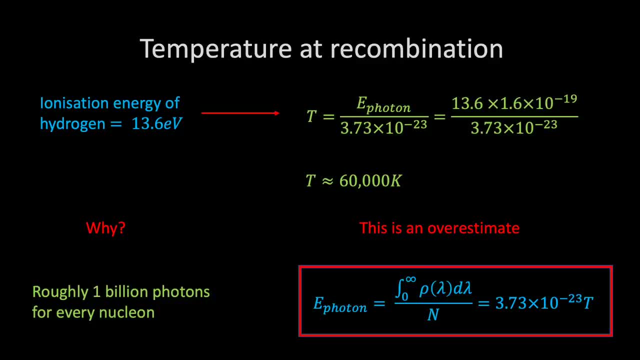 for every nuclear particle in the universe. We will discuss this in a bit more detail later, but for now the key point is that even if the average photon energy is well below 13.6 electron volts, because there are so many photons, there will still be plenty of photons in the high energy tail of 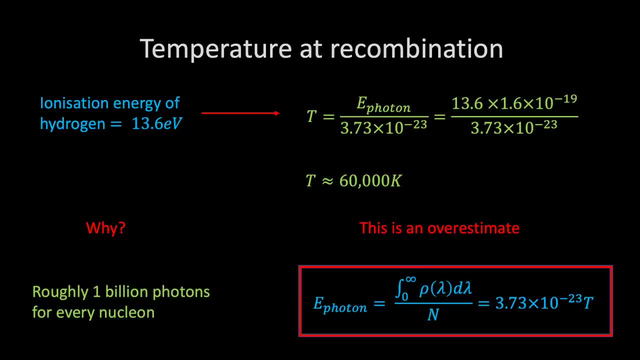 the Planck distribution with enough energy to ionize hydrogen. A more detailed calculation, which factors in the photon to nucleon ratio, finds that the temperature of recombination is in fact closer to 3000 kelvin. The details of this calculation are beyond the scope of this video. 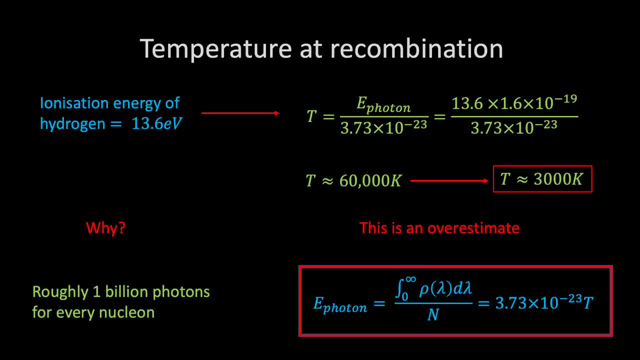 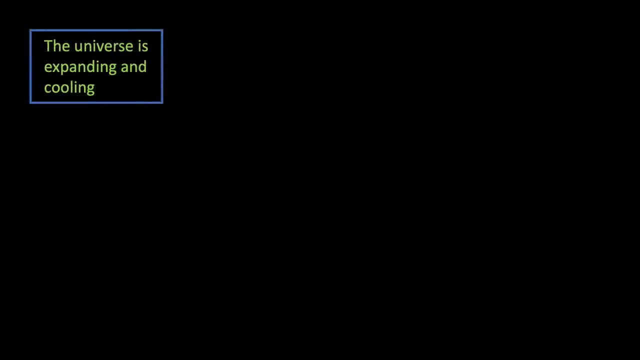 but for those who are interested, I've put some links in the video description. So let's just recap where we are at. The big bang theory predicts that the universe is expanding and cooling and therefore we know that during the early phases of the universe, the temperature 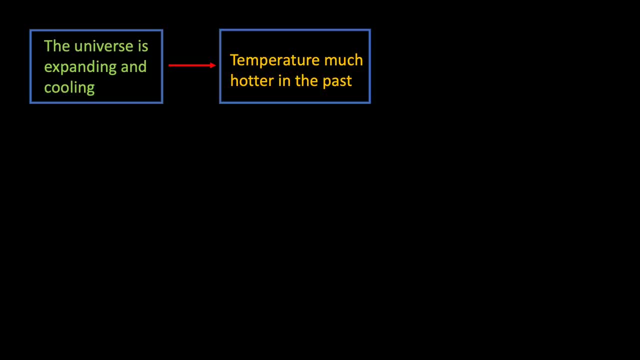 must have been much hotter than the present 3k temperature of the microwave background radiation. And we've just seen that during the earliest phases of the universe, when the temperature was over 3000k, the universe would have been opaque to radiation, Since decoupled nuclei and electrons would have absorbed and scattered photons and furthermore, 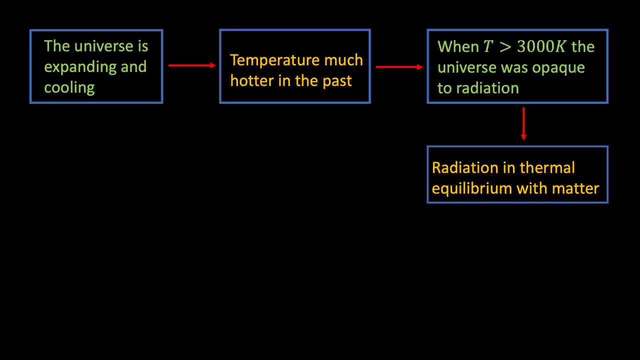 the radiation would have been in thermal equilibrium with the matter content of the universe. As the universe continued to expand and cool, at some stage the temperature would have dropped below 3000k and at this point the electrons and nuclei were able to combine to form neutral atoms. 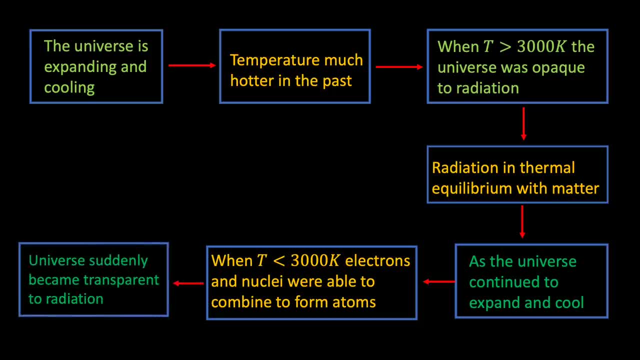 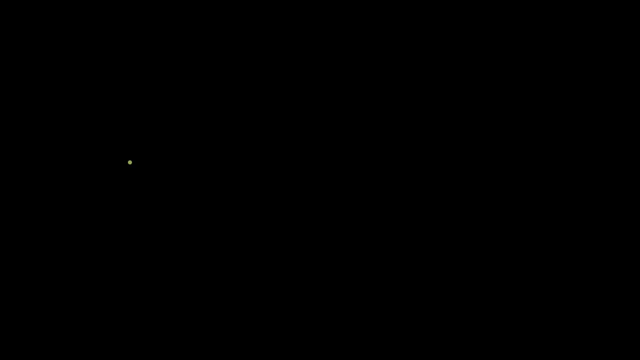 and the universe suddenly became transparent to radiation. So what has happened to these photons since then? To answer this question, we need to understand how light is affected by an expanding universe. Observational evidence for the expansion of the universe relies on the Doppler effect. 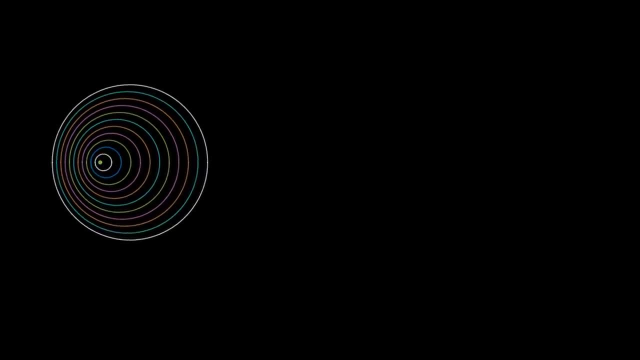 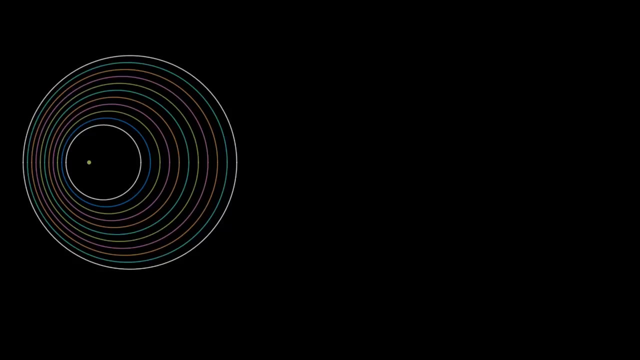 which tells us that the wavelength of light emitted from a source that is moving should be shifted. To see this, suppose that a wave crest leaves a light source at regular intervals separated by time period t. If the source is moving at a velocity of t, it's going to be a wave crest. 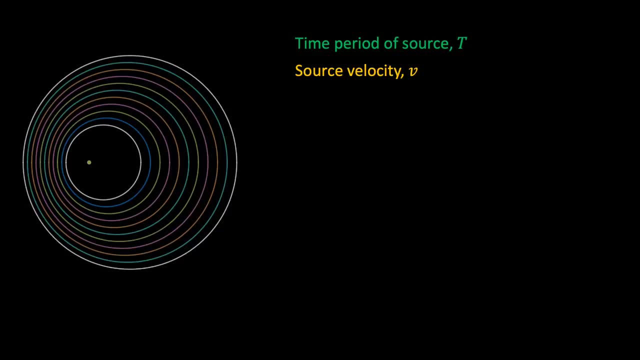 v away from the observer, then during the time between successive crests, the source moves a distance vt. This then increases the time required for the wavecrest to get from the source to the observer by an amount vt over c, where c is the speed of light. Thus, 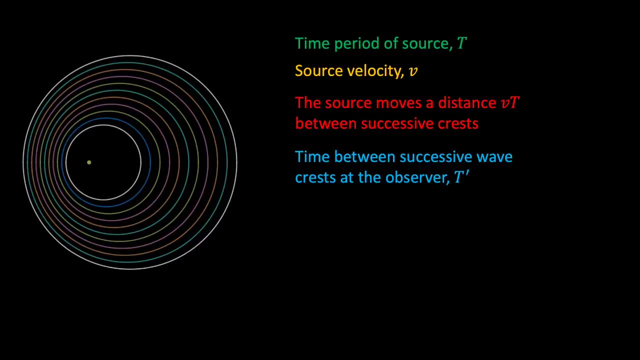 the time between successive wavecrests at the observer. t prime is given by. t prime equals t plus vt over c. We can write an expression for the wavelength of the light upon emission as lambda equals ct, and then the wavelength when the light arrives is lambda prime equals. 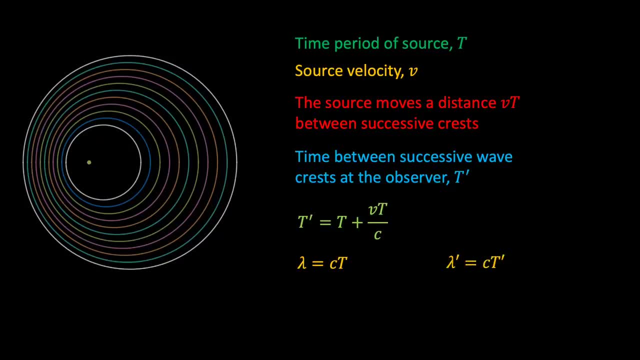 ct prime. Thus we see that the ratio of wavelengths can be written as lambda. prime over lambda equals 1 plus v over c, which corresponds to a shift in wavelength towards the red end of the spectrum. If the source was moving towards the observer instead, we would simply: 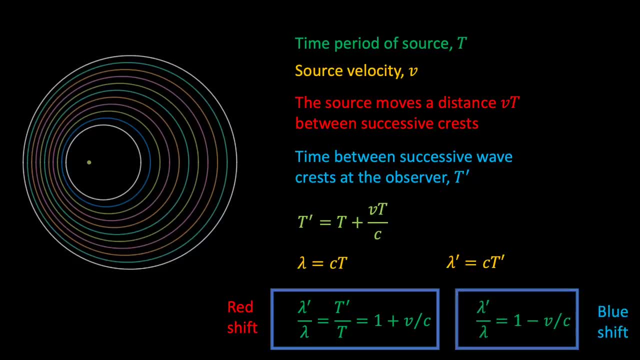 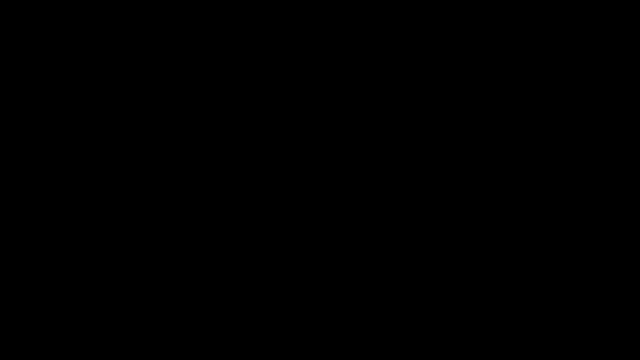 replace v with minus v and we would then have lambda prime over lambda equals ct. Next, consider a light wave travelling between two galaxies. The separation between the galaxies equals the light travel time multiplied by the speed of light and the increase in separation. 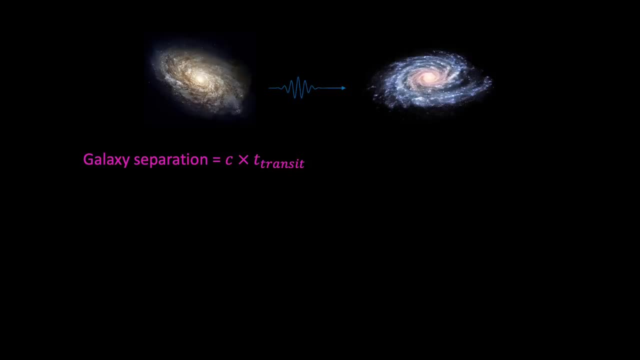 during the light transit time equals the light transit time multiplied by the relative velocity of the galaxies. If we calculate the fractional increase in separation z, we have that z equals the increase in separation in the light transit time to one minus v over, divided by the mean separation during the increase, and this is equal to v times t transit divided by. 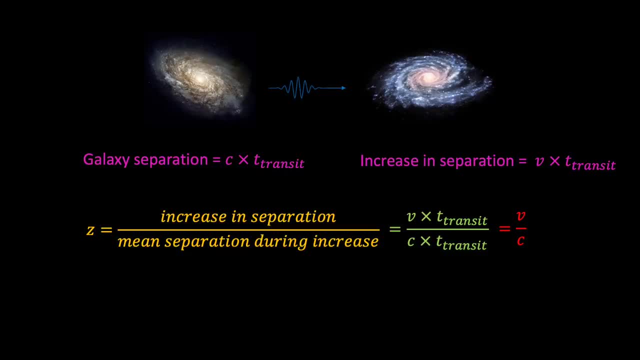 c times, t transit, which simply equals v over c, and we see that the transit times cancel out, and this is the same ratio that we saw earlier for the fractional increase in wavelength of light during this time, Therefore, the wavelength of any light ray increases in proportion to the 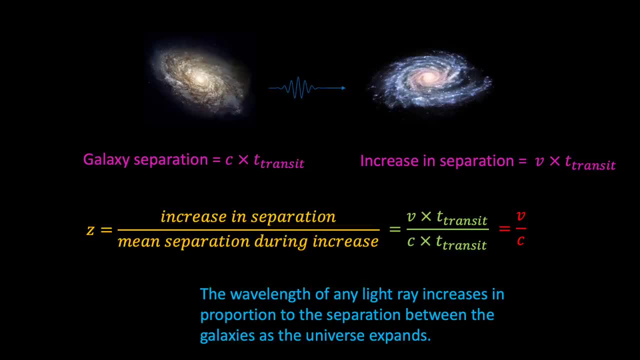 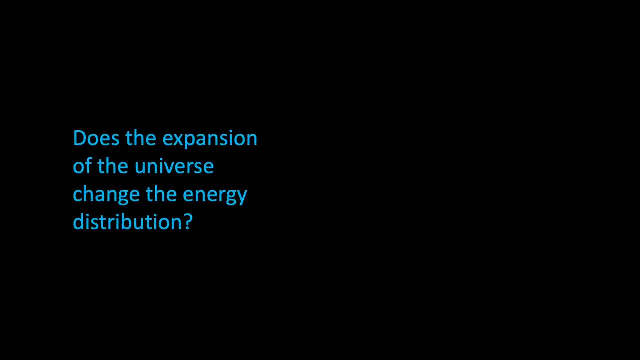 separation between the galaxies as the universe expands. If the wavelengths of light appear to stretch, then we must conclude that the universe itself has also grown by the same amount. So the question we need to answer is whether the expansion of the universe and the subsequent increase of wavelength would change the energy distribution of radiation, or will the radiation? 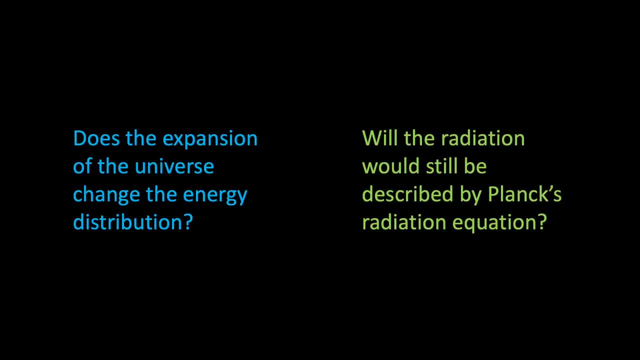 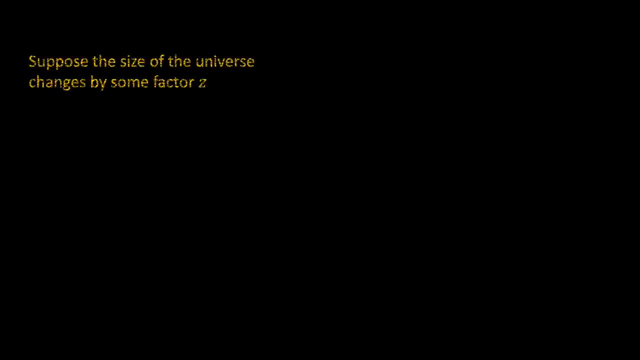 still be described by Planck's radiation law, even though the radiation is no longer in thermal equilibrium with the matter of light? To answer this question, suppose the universe increases in size by some factor z, As we've just seen. the wavelength will also increase by the same factor As a result of the expansion, the new energy. 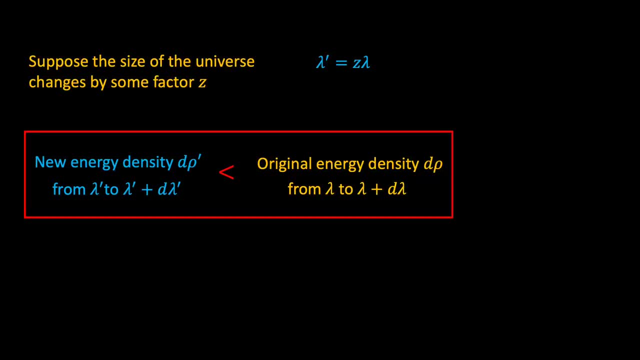 density will be less than the original energy density for two different reasons. Firstly, since the volume of the universe has increased by a factor z cubed, as long as no photons have been created or destroyed, the number of photons per unit will increase by a factor z cubed. 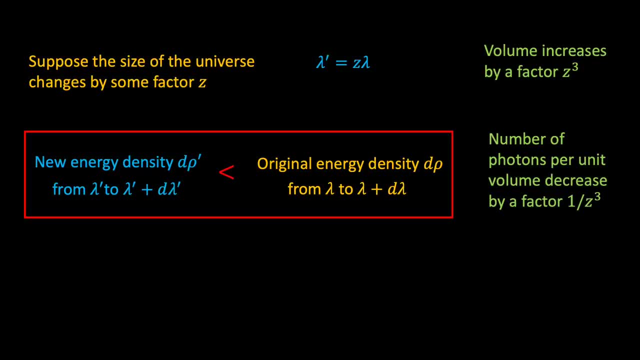 Secondly, we know that the energy of each photon is inversely proportional to its wavelength and therefore, if the wavelength increases by a factor of z, the energy of the photon will decrease by a factor of one over z. It then follows that the energy density is decreased by an overall factor. 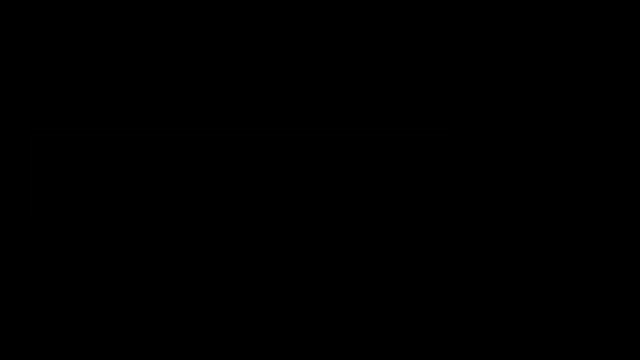 of one over z to the power of four, And therefore we can write the new energy density, d rho prime as the following equation: If we then rewrite this in terms of the new wavelength lambda prime, we get this light blue expression And we see that this is exactly the same as the old equation for the energy density, except the temperature. 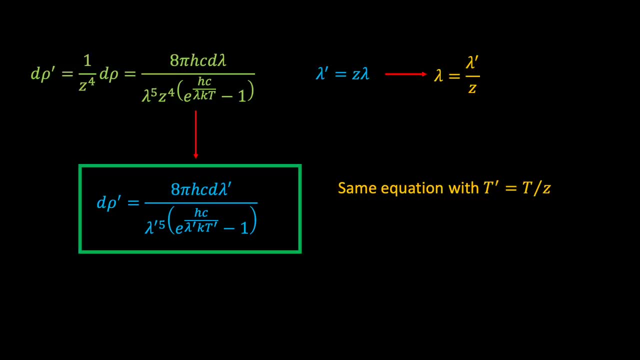 T has been replaced by a new temperature. T prime equals T over z. Thus we see that the radiation filling the universe would continue to be described precisely by the Planck radiation law as the universe expanded, But with the temperature 10 over z, which continues to be equal to what we believe is the energy density of the photon. 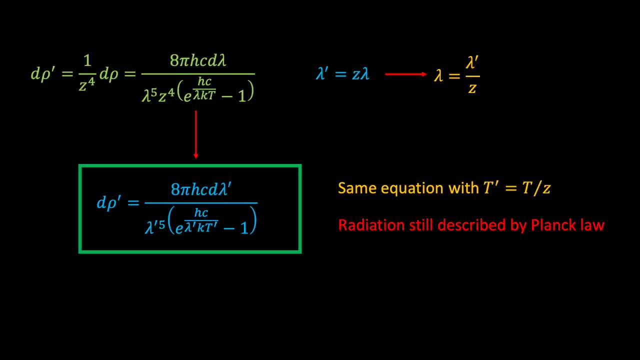 that decreases in inverse proportion to the scale of the expansion, and this is true even though the radiation is no longer in thermal equilibrium with the matter content of the universe. The only effect of the expansion is to increase the wavelength of each photon in proportion to the size of the universe. 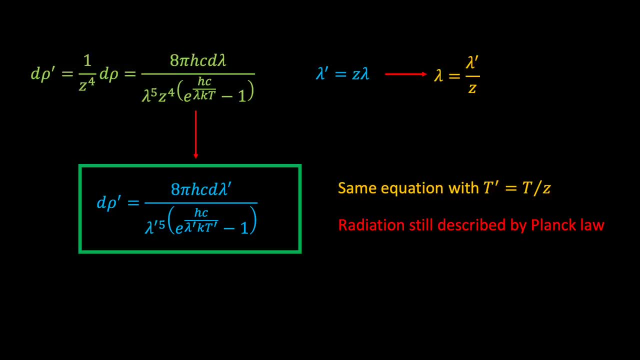 Now, if you recall, Penzias and Wilson found a temperature of around 3 Kelvin, which is a factor of 1,000 times smaller than the 3,000 Kelvin minimum temperature required to keep matter and radiation in thermal equilibrium, and therefore, according to our previous analysis, we see that the universe should. 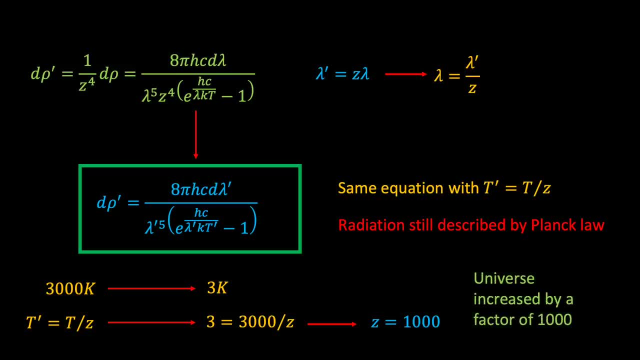 have expanded by a factor of 1,000 since this time. If this interpretation is indeed correct, then the 3 Kelvin microwave background radiation is by far the most ancient signal received by astronomers when looking at the universe, long before stars formed and light was emitted from the most distant. 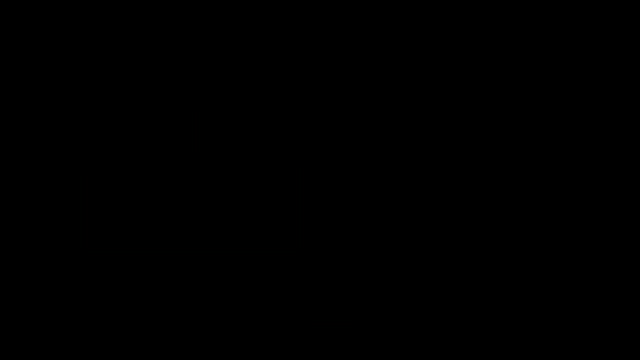 galaxies that we can see. It therefore became a matter of extreme urgency to measure the energy density of the microwave radiation at other wavelengths, so that the wavelength energy profile could be compared with the Planck radiation law. After all, Penzias and Wilson had only measured the intensity. 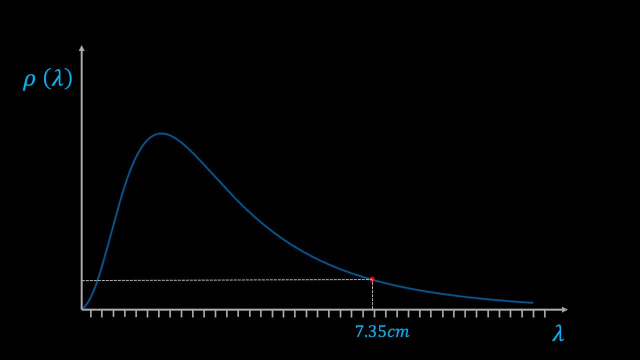 of microwave radiation at a wavelength of 7.35 centimeters, whereas we know from Wien's displacement law that the peak intensity of microwave radiation at 3 Kelvin is in fact at a wavelength of roughly 0.1 centimeters Around the same time that Penzias and 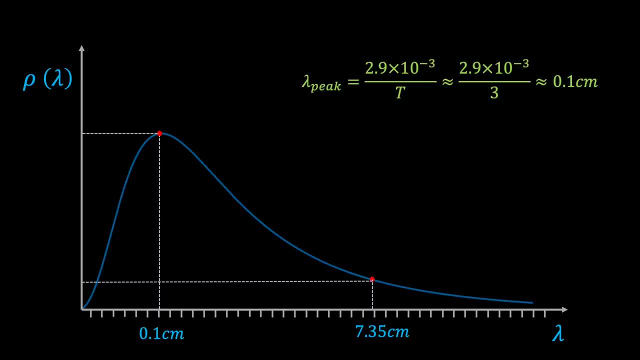 Wilson detected their 7.35 centimeter radiation. two physicists, PG Roll and DT Wilkinson, also mounted a search for microwave radiation using a small low-noise antenna on the roof of the Palmer Physical Laboratory at Princeton. Only their antenna was tuned to 3.2 centimeter. 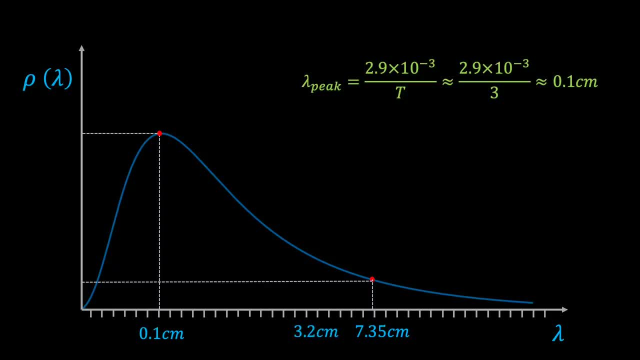 wavelength microwaves. When they analyzed their results, they found that the microwave radiation was at a wavelength of 0.1 centimeters. This means that the microwave radiation was at a wavelength of 0.1 centimeters. They found that the intensity of their microwave 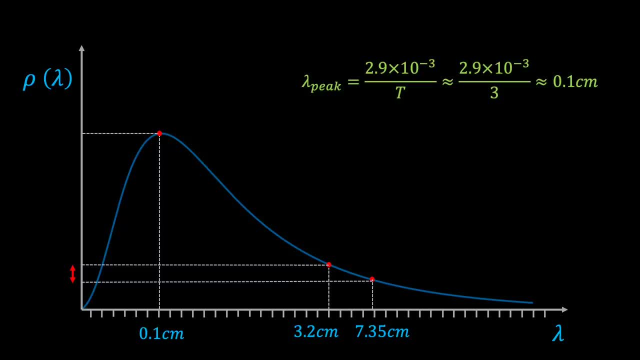 radiation at this slightly shorter wavelength was greater than the intensity at 7.35 centimeters, by the exact ratio predicted by the Planck radiation law. Over the years that followed, the microwave radiation was measured by several different groups of astronomers at a range of wavelengths from 73.5 centimeters all the way down to 0.33 centimeters, and every one 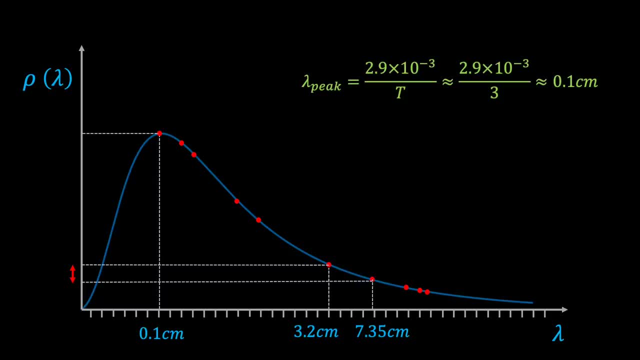 of these measurements was consistent with the Planck distribution, corresponding to a temperature of close to 3 Kelvin. However, as you might have noticed, all these measurements are at wavelengths longer than the peak wavelength expected for this temperature, In order to verify that the radiation really is described by the Planck distribution. 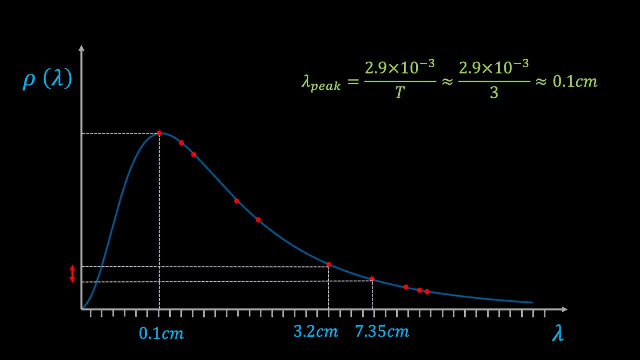 and not just some long wavelength approximation. it was necessary to check that the intensity really does fall off at short wavelengths, as predicted by the Planck radiation law. However, the trouble with the Planck radiation law is that it is not necessarily the same as the Planck radiation law. 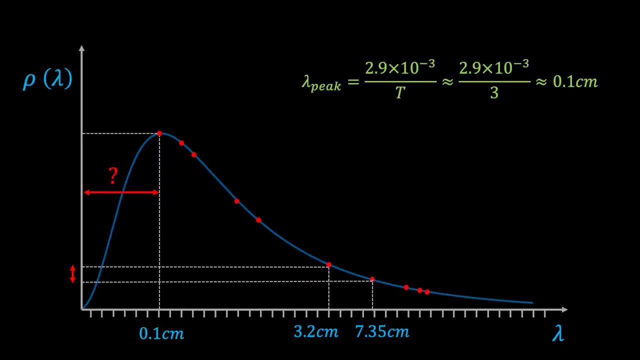 The problem with measuring shorter wavelengths is that the atmosphere of our planet gets in the way For wavelengths less than around 0.3 centimeters. the atmosphere becomes increasingly opaque due to the absorption of light by ozone, oxygen and water vapour. So how do 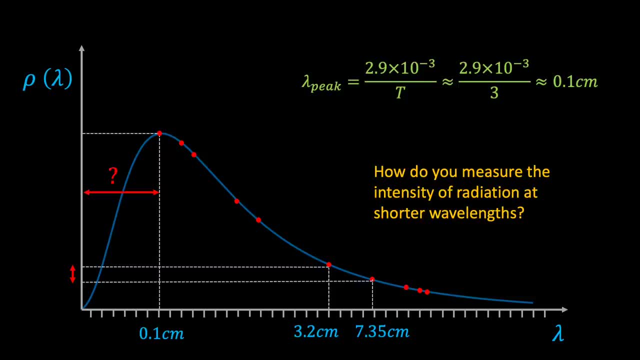 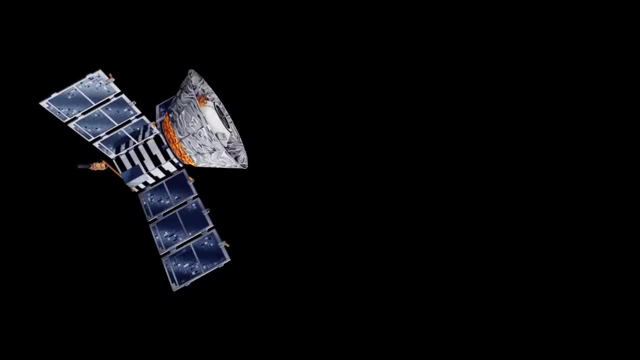 you measure the intensity of radiation at short wavelengths? Well, the answer is that you find a way of placing your detector above the Earth's atmosphere. Initially, this was achieved using rockets and balloons, allowing the Planck radiation law to work. if yourβ. 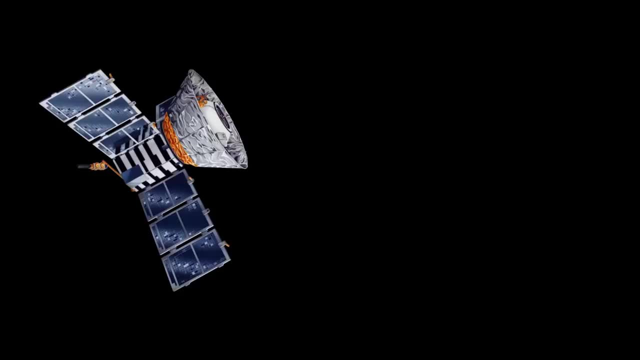 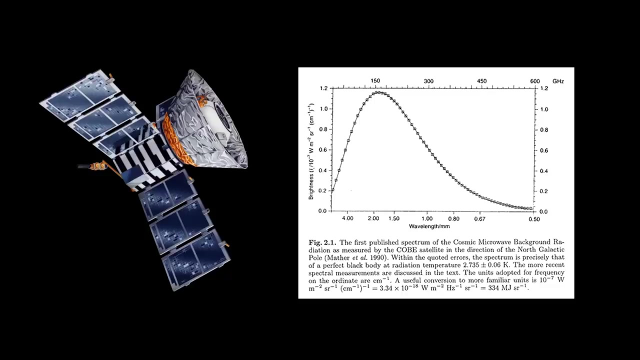 law to be confirmed to wavelengths as low as 0.06 cm. but the great turning point came in 1989 with the launch of the Cosmic Background Explorer, or COBE for short, which was able to provide detailed measurements of the background radiation intensity at a range of short wavelengths. The 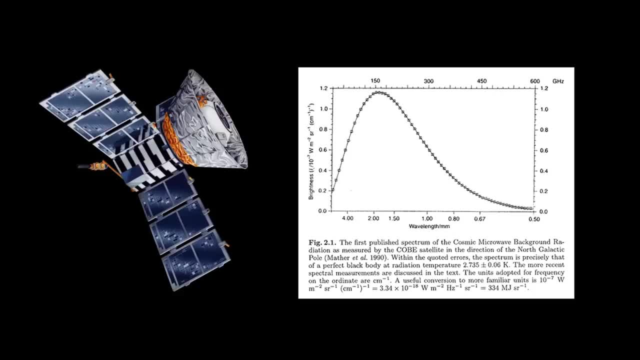 results, as you can see in the graph plot, were astounding, confirming that the background radiation perfectly fits the Planck distribution predicted by a Big Bang model and, furthermore, that the present temperature of the microwave radiation has a value of 2.735 Kelvin. 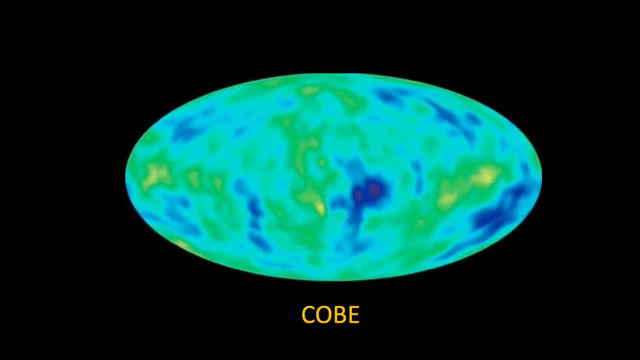 But the excitement didn't stop here. The COBE satellite had also been designed to measure very faint irregularities in the intensity of the cosmic radiation. It was thought that there might be small fluctuations in the intensity caused by the actual lumpiness of the universe, either at 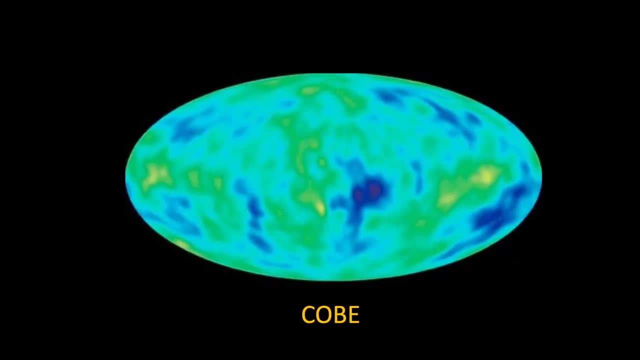 the time the radiation was emitted or since then. For example, galaxies in their early stages of the cosmic radiation had a very faint irregularity in the intensity of the cosmic radiation. The COBE satellite's development might show up as hotspots in the sky with slightly higher 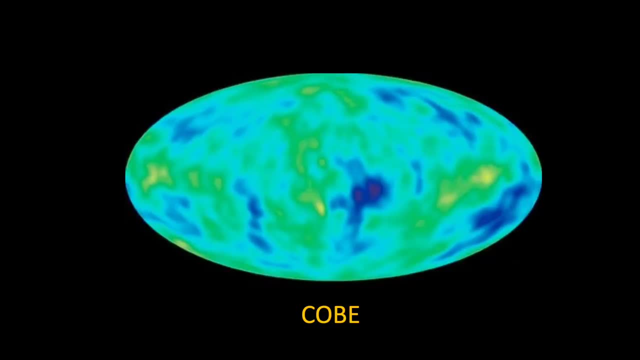 temperatures than the average 2.735 Kelvin. Finally, in 1992, the COBE scientists announced that they had detected small non-uniformities in the microwave radiation at a level of one part in 100,000.. By way of comparison, if the Earth's surface was smooth to one part in 100,000,. 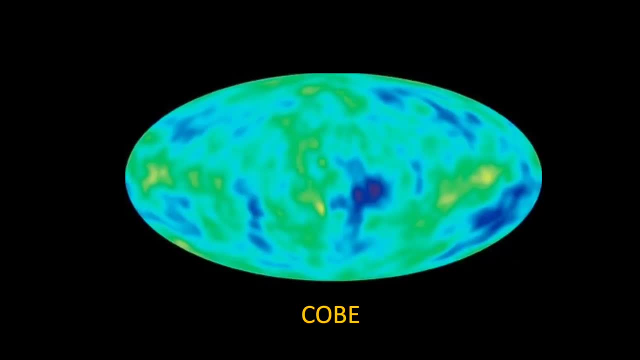 then the highest mountain would be just 100 meters tall. However, the clumps causing the temperature fluctuations detected by COBE were much too large to be attributed to individual galaxies. In order to observe the beginnings of galaxies and galaxy clusters, it would be necessary to measure temperature fluctuations with a far 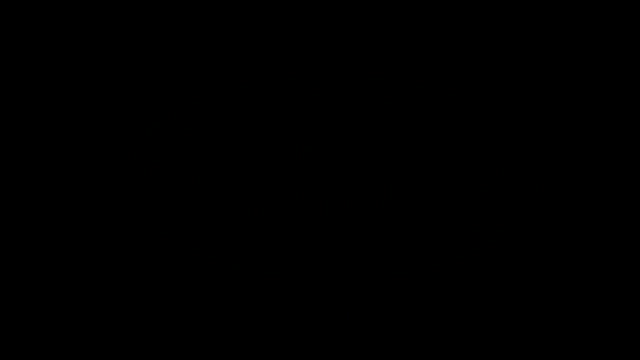 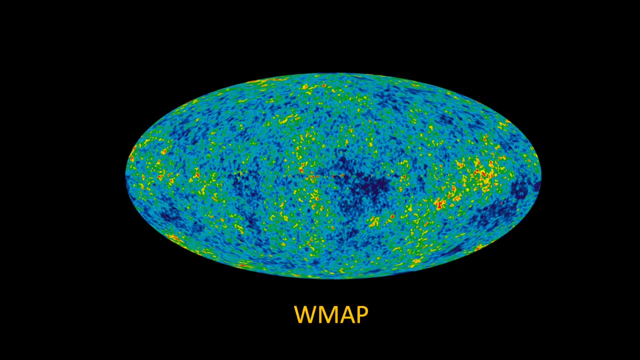 higher resolution than could be achieved with the COBE satellite. Thankfully, over the past 30 years, new and improved measurements have helped to clarify the situation. On June 30, 2001,, NASA launched a follow-up mission to the Earth and it was a success. The COBE satellite was a 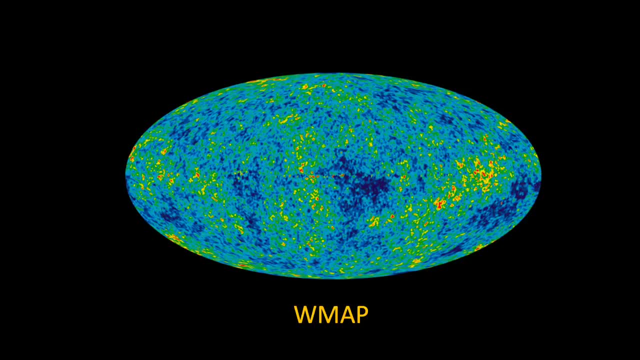 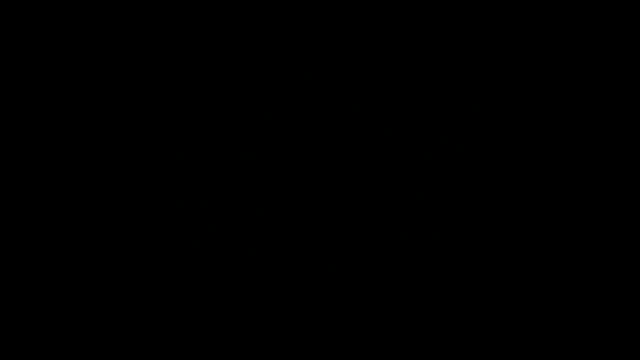 satellite that was built into COBE, called the Wilkinson Microwave Anisotropy Probe, or WMAP, which was able to significantly improve on the resolution of the COBE satellite. And then, in 2009,, the European Space Agency launched the aptly named Planck satellite, which mapped 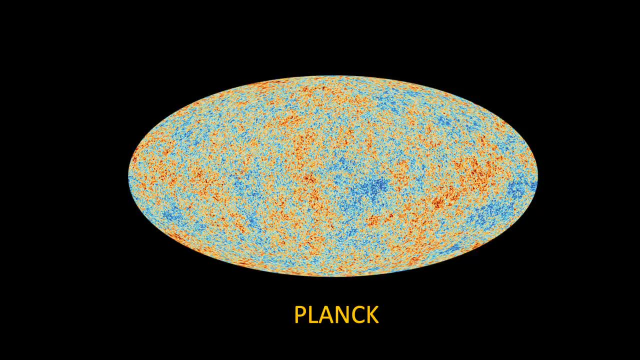 the irregularities with extremely high sensitivity and small angular resolution, again confirming the Planck distribution of thermal radiation. as well as providing valuable information about the fine-grained density irregularities, The Planck satellite was also designed to measure the temperature fluctuations in the 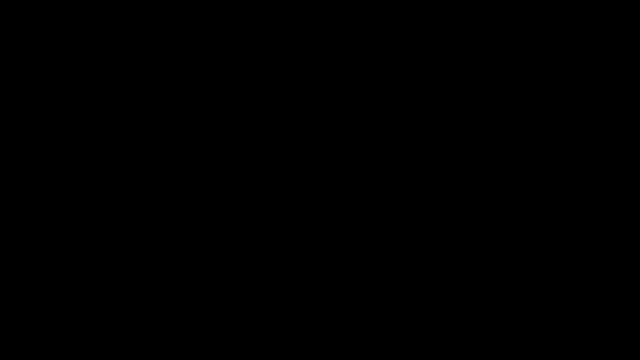 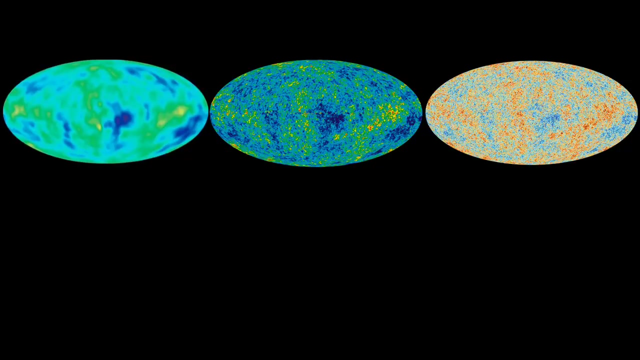 irregularities in the early universe. What is quite remarkable is that these irregularities can be analysed to extract all sorts of useful information about the universe. In particular, they can be used to determine how the first stars and galaxies formed. how much normal matter is in 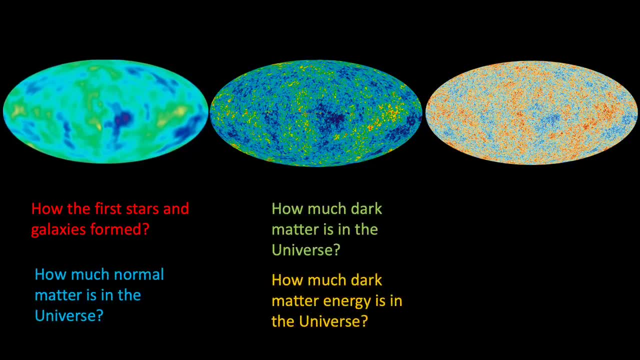 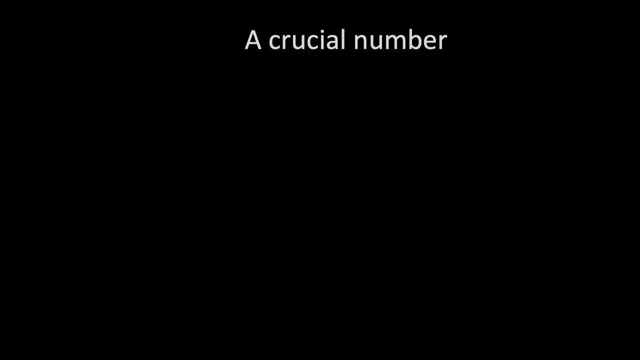 the universe, how much dark matter and dark energy is in the universe, as well as the overall shape and curvature of the universe. Each of these fascinating lines of inquiry will require their own video, and I will therefore leave these dangling carrots here for now. Instead, I'd like. 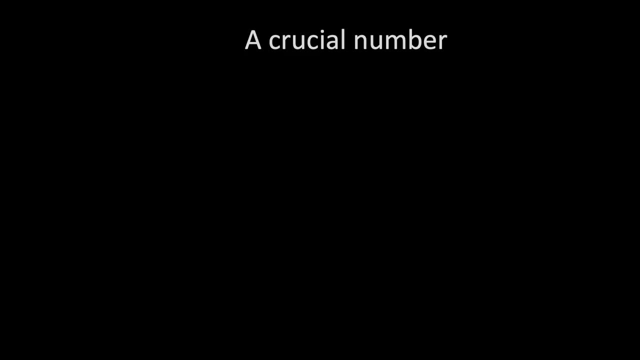 to focus on another important cosmological insight that we can draw from our knowledge of the temperature of the cosmic microwave background radiation. As we've already seen, the number of photons per unit volume is directly proportional to the cube of the temperature. So we see that at 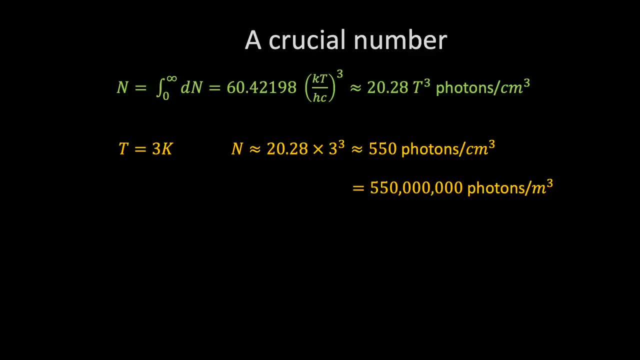 a temperature of 3 Kelvin, there are roughly 550 million photons per cubic metre. However, based on estimates of the critical density of the cosmic microwave background radiation, we can see that of the expanding universe, the density of nuclear particles is believed to be somewhere between 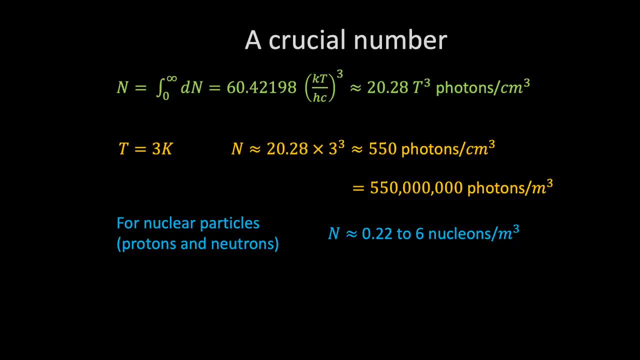 0.22 and 6 per cubic metre. In other words, according to our current best estimates for the nuclear density of the universe, there were roughly 1 billion photons for every nuclear particle in the universe today. Furthermore, it's believed that this ratio has been constant. 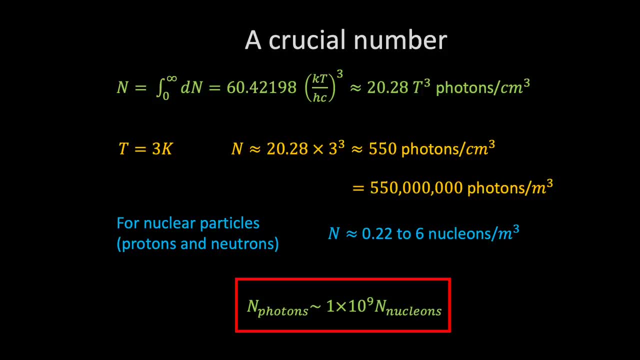 ever since the temperature of the universe dropped below 3000 K. Now this ratio is, in a sense, the most important quantitative conclusion that can be made. to determine the temperature of the universe, We can be drawn from the data of the cosmic microwave radiation, as it allows us to precisely determine 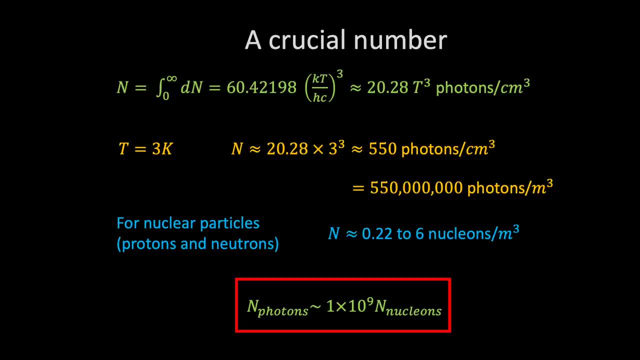 when the matter content of the universe started condensing to form stars and galaxies. In fact, the formation of stars and galaxies could not have begun until the cosmic temperature became low enough for electrons to be captured by nuclei to form atoms. To understand why, let's delve a. 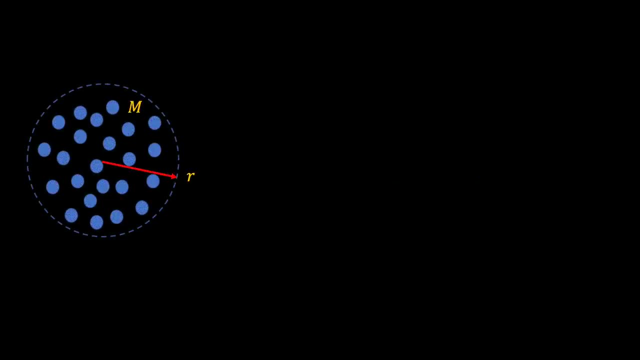 little deeper. Consider a spherical region of space containing matter with total mass m. In order for clumping to occur, it is necessary for the gravitational force of attraction to overcome the outward pressure caused by thermal motion of matter and the associated radiation. At any given density and pressure, there is a minimum mass which is susceptible to gravitational. 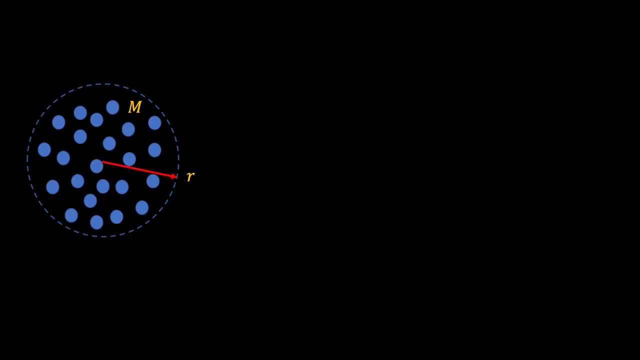 clumping. This is known as the Jeans mass. For a clump of matter to form a gravitationally bound system, it is necessary for its gravitational potential energy to exceed its internal thermal energy. The gravitational potential energy of a clump of radius R and mass m is of order. 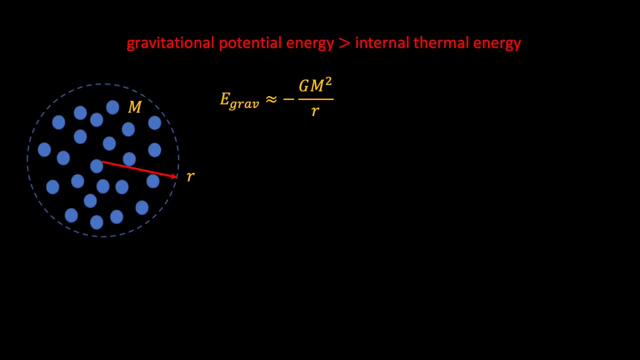 minus gm, squared over R, which simply follows from Newton's universal law of gravitation. On the other hand, the internal energy is proportional to the pressure times the volume, and so we can write this as p times R. cubed, You can check that this does indeed have the required units of energy. 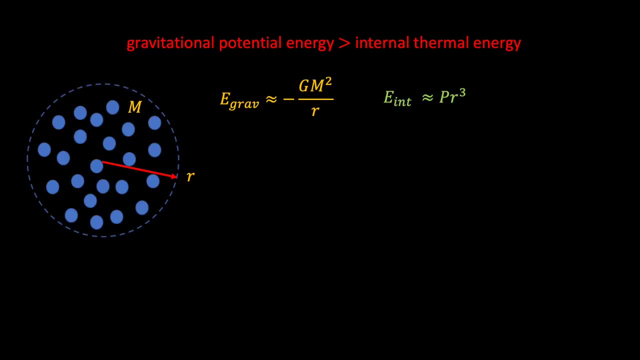 and so we see that in order for gravitational clumping to occur, we require that gm squared over R is greater than pr cubed. We can combine the definition of density with the volume of a mass of r cubed equals 3m over 4 pi rho, and if we then substitute this into the clumping, 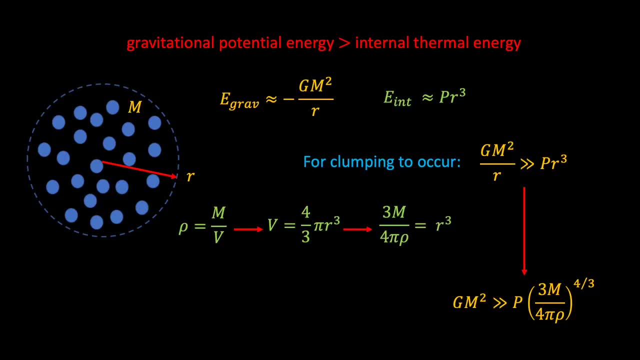 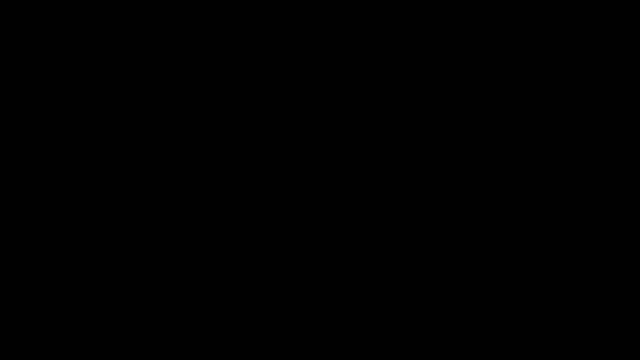 condition, we find this yellow expression. If we then rearrange for m, we find an approximate expression for the Jeans mass in terms of the pressure and density. We can then use this equation to estimate the Jeans mass just before recombination occurred, As we have. 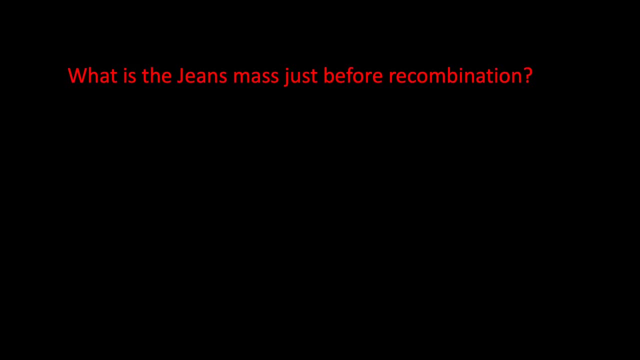 already established, the temperature at recombination was around 3000 Kelvin, in which case the energy density is 3.83 times 10 to the 14 kiloelectronvolts per cubic meter. We can rewrite this as an equivalent mass density by converting the energy into its mass equivalent, using Einstein's famous 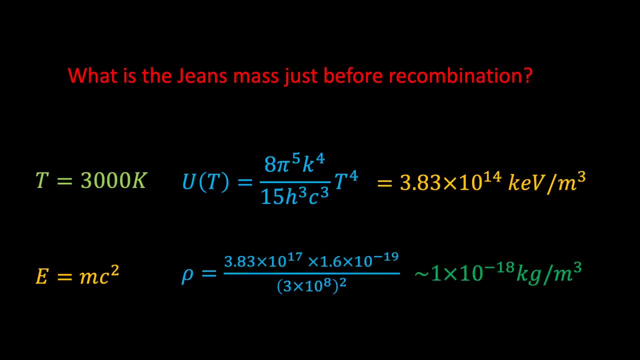 equation equals mc squared. If we do this, we find that just before recombination the mass density would have been around 1 times 10 to the minus 18 kilograms per meter cubed. Our next task is to work out an equation for the pressure prior to recombination. 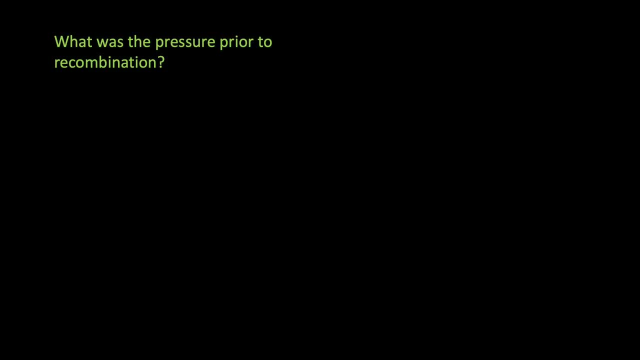 During this time, the outward pressure counteracting gravitational collapse would have been dominated by so-called radiation pressure. As you know, pressure is defined as the force per unit area or rate of change of momentum per unit area. Next consider photons bouncing back. 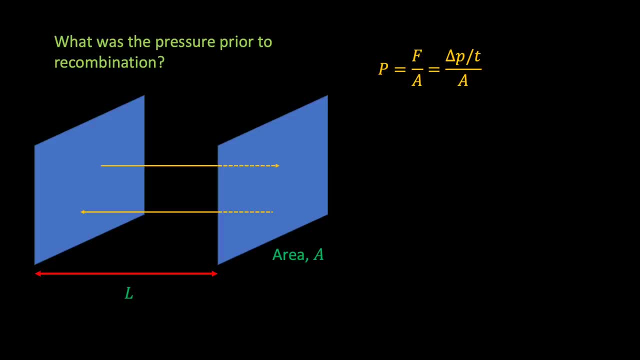 and forth between two parallel mirrors of area A and separation L. If we assume a photon moving to the right has momentum p, then when it reflects off the mirror and moves to the left, it will have momentum minus p. Therefore the change in momentum is equal to 2p each time the photon bounces off the mirror. 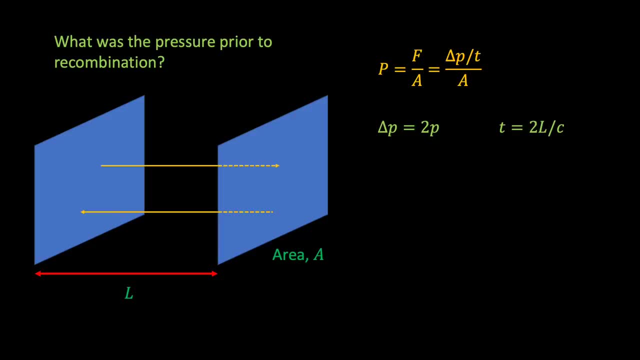 These bounces occur on a given mirror every 2l over c seconds, and therefore we see that each photon's contribution to the pressure is given by. p equals e over v, And so if we add up all the photon energies, we see that the pressure will simply be equal to the energy density. 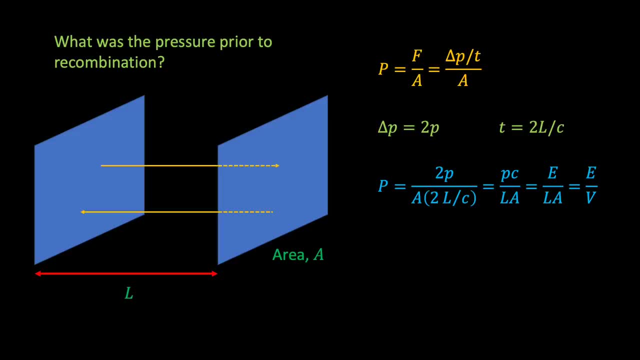 But wait, we have to be a little bit careful, because we have forgotten that photons will be moving in all directions. Because the photons will be moving randomly, there will be no preferred direction and therefore we have to average over the three coordinate directions- x, y and z, as is standard. 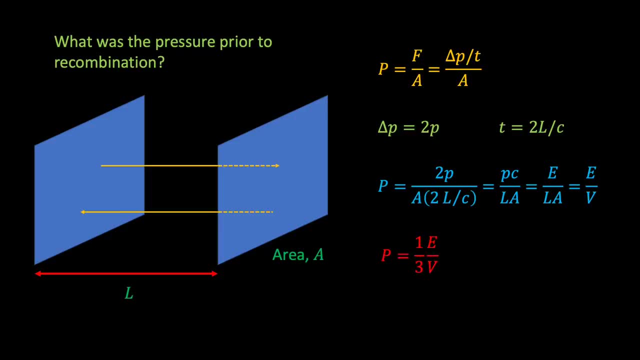 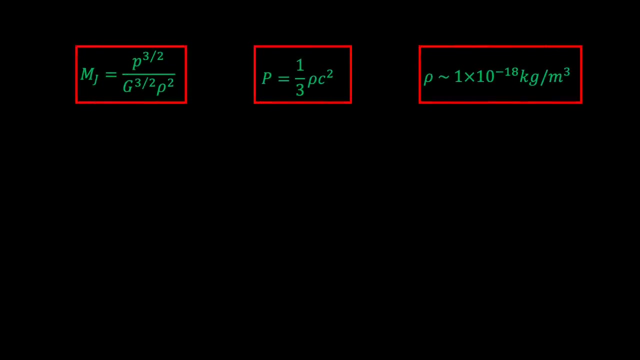 when dealing with gas pressure, And so the pressure becomes: p equals a third times e over v. If we then write this in terms of the mass equivalent, using e equals mc squared, we get that p equals a third rho times c squared. If we now combine all of our previous calculations, 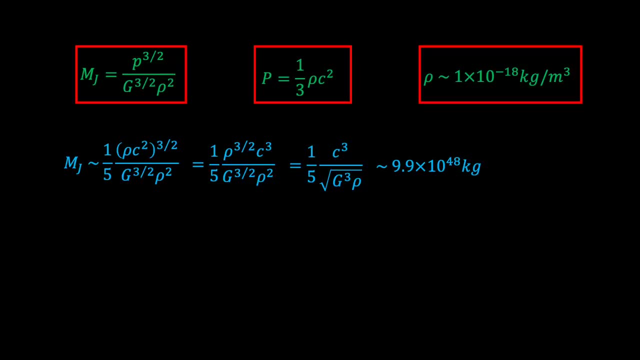 we see that just prior to recombination, the gene's mass was roughly 9.9 times 10 to the power of 48 kg, which we can write as 5 times 10 to the power of 18 solar masses, where one solar mass is equal to the mass of our sun, which is around 2 times 10 to the 30. 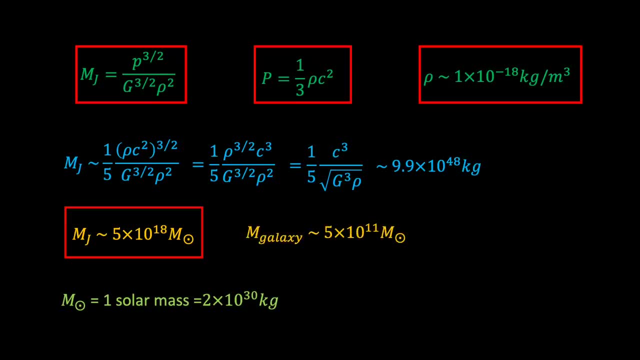 kg. By way of comparison, the mass of our galaxy is around 5 times 10 to the 11 solar masses, and so we see that before recombination, the gene's mass was over a million times the mass of a large galaxy. 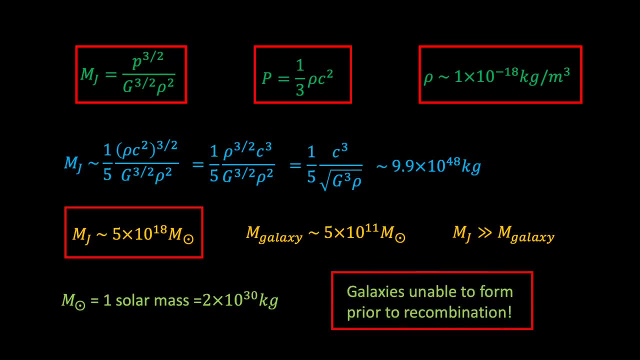 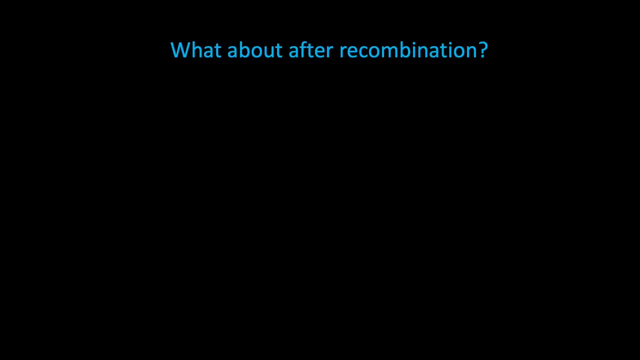 And therefore neither galaxies or clusters of galaxies could have formed at this time. So what about after recombination? Well, as we've already seen, at this stage the universe became transparent to radiation and therefore the photons would have essentially stopped contributing to the outward pressure. And since, as we've seen, there are roughly one. 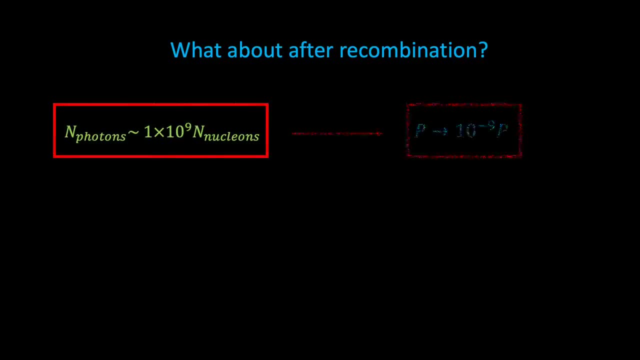 billion photons for every nuclear particle. the pressure would have dropped by a factor of one billion and therefore the gene's mass would have reduced by a factor of one billion and also the current of those potential galaxies would have been reduced by a factor of 10. 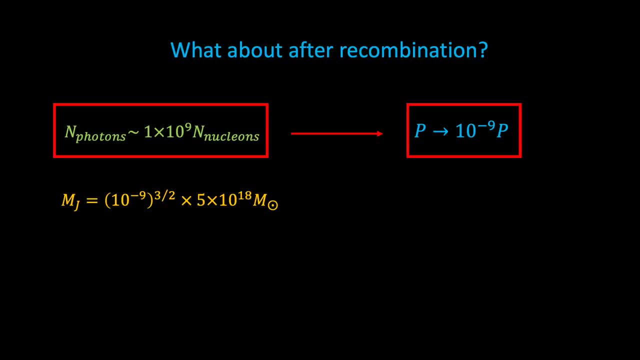 to the minus 9, raised to the power of 3 over 2.. And so we see that the gene's mass would have dropped to around 1.6 times 10, to the power of 5 solar masses, which is about a millionth the mass of a galaxy. From this point onwards, the pressure of radiation could.